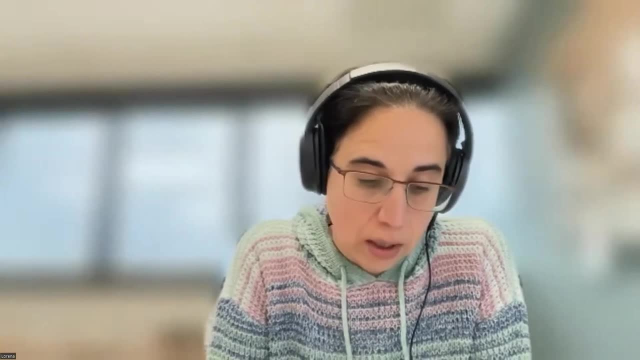 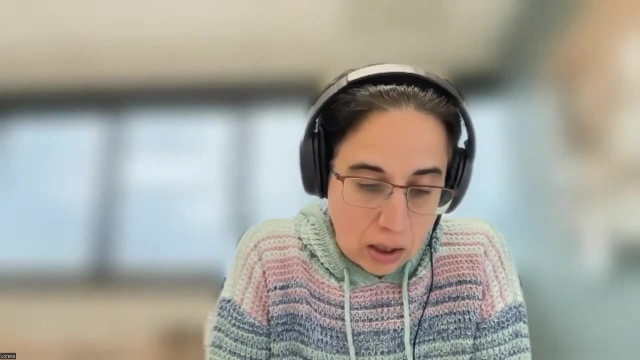 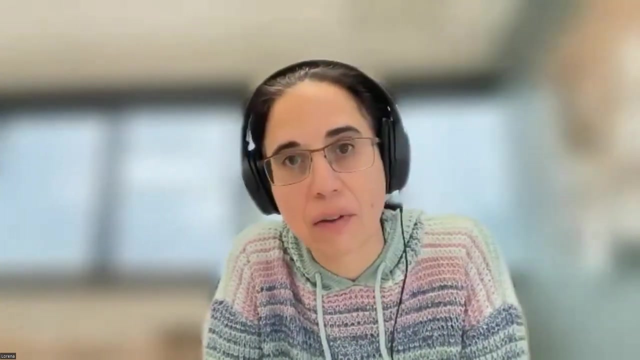 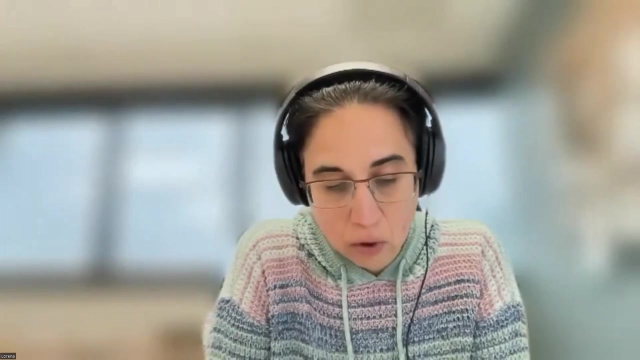 In 2020, he continued. He continued as a postdoctoral researcher and geology instructor in Louisiana State University And in 2022, he was hired by Ellington Geological Services as a staff biostratigrapher. He has a wide range of interests in his research that include encretaceous mass extinction, early paleogene hyperthermal events. 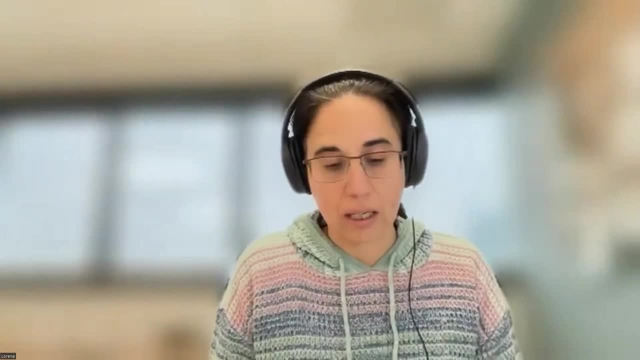 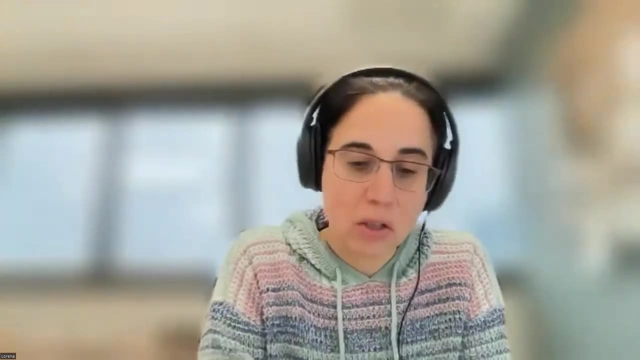 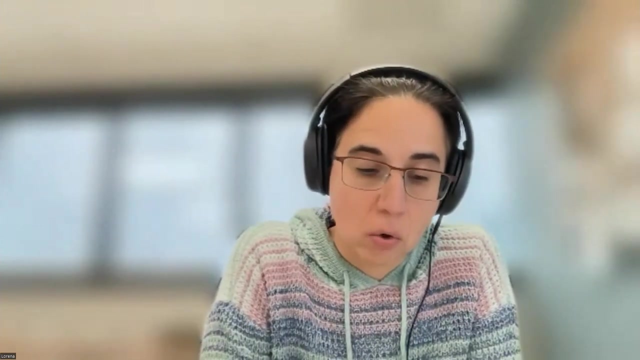 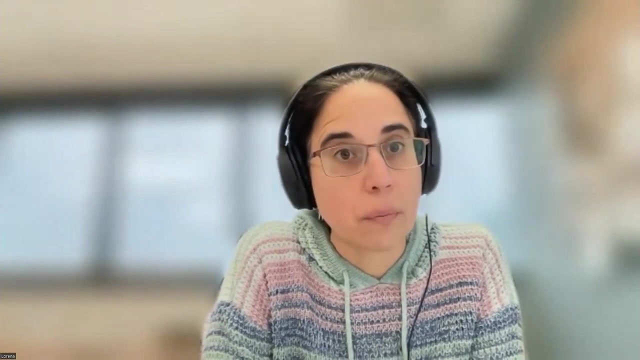 cenozoic plant evolution and the reconstruction of of Holocene climate using pollen records. I'm really excited today to introduce Van, who's going to give a presentation where he will be showing some results from a STAR-Ellington collaboration that we initiated last year in the onshore lower Wilcox group. So with that I'm going to pass the baton to Van Van. the floor is yours. 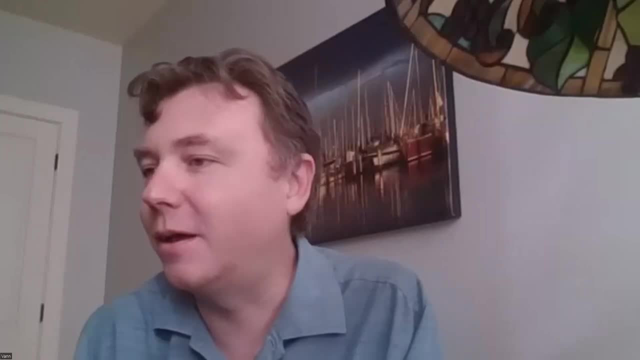 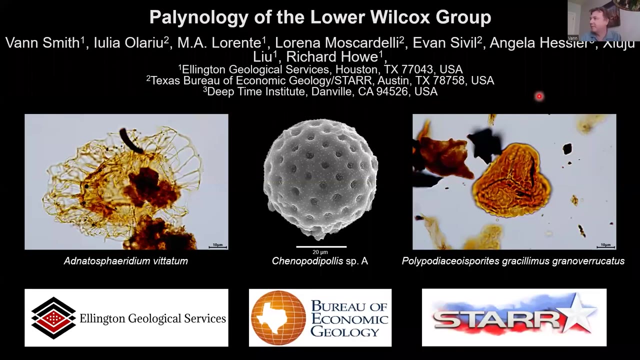 Okay, thank you, Lorena. I will share my screen, So can everyone see this? Yes, it's working, Okay cool, Okay. good morning everyone. First, I'd like to say that it's an honor to be invited to be a speaker for the Bureau And I hope you find the talk interesting. We have some great collaborators here. 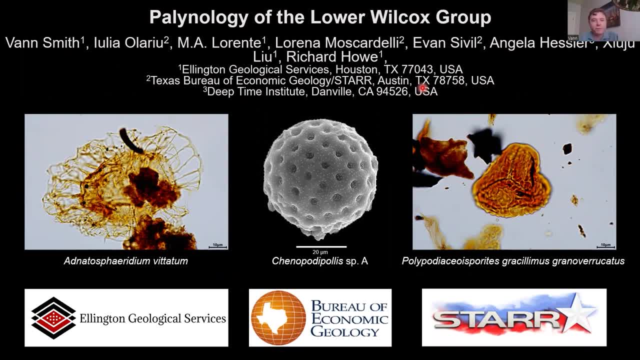 I'm going to be mainly focusing on the palynology, but there's also a lot of work being done on the, the chemistry, the geochemistry and the lithostratigraphy and other aspects of this research into the lower Wilcox group. 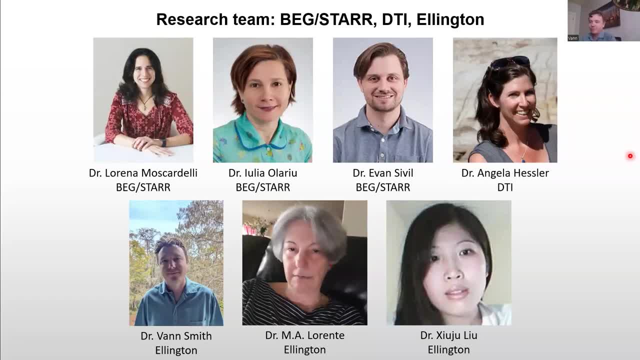 So to a brief introduction to our research team. you guys probably know most of these people already, but I wanted to just mention them briefly. So Dr Lorena, who introduced me, We have Dr Iulia and Sibyl, all at BEG STAR, Dr Anita Hartler at the Deep Time Institute and myself, Tania Llorente and Khidri Liu at Ellington. 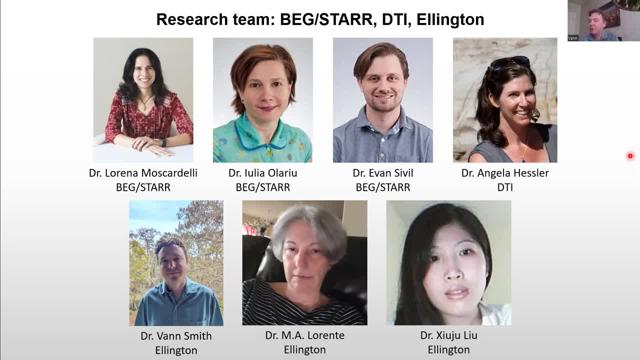 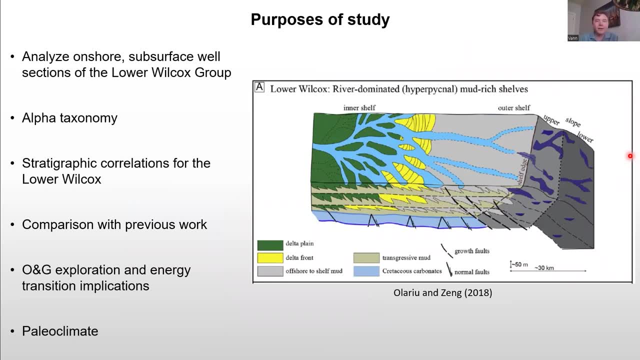 And Rich Hao has done done some work for us with the nanos as well. For the purposes of this study, we are looking at two subsurface wells in the lower Wilcox group onshore And as a palynologist I had a particular interest in doing some alpha taxonomy, which basically just means the description and describing. 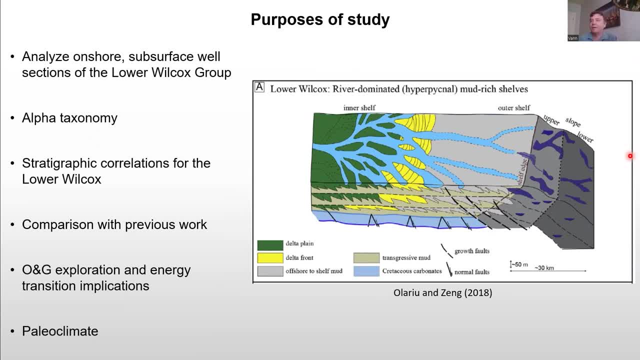 how, how we name different species and that kind of thing, And I'll explain that a little more detail later. We are also interested in stratigraphic correlations for the lower Wilcox, both biostratigraphic, chemostratigraphic, lithostratigraphic. 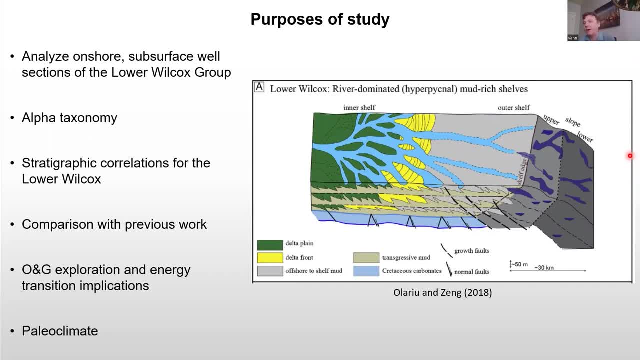 And also to compare it with previous work done on outcrop onshore and the deepwater. So there's important applications here in in oil and gas exploration. The deepwater Wilcox is an important hydrocarbon reservoir and palynology is often used for the biostratigraphy. 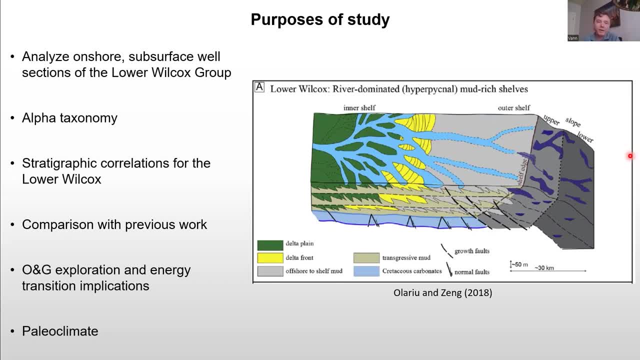 and particularly because it's often nanofossil and forams are not as useful just because they're diluted- And also has important implications for energy transition, like carbon capture and storage, And it also has implications for paleoclimate. There's been a lot of previous work done in the lower Wilcox. 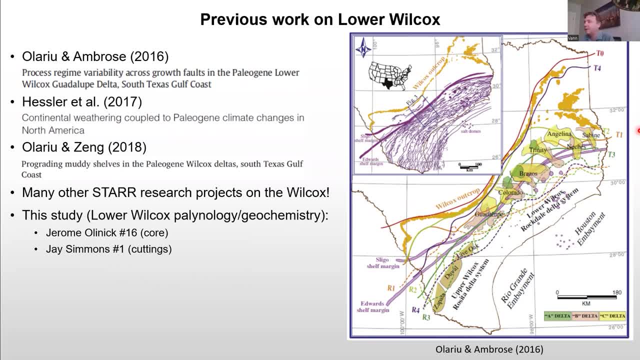 including by some of the collaborators on this project that I'll briefly mention. So this map here is showing the delta system in the Wilcox and then the Wilcox outcrop. So it outcrops sort of parallel to the coastline here and then dips down into the subsurface. 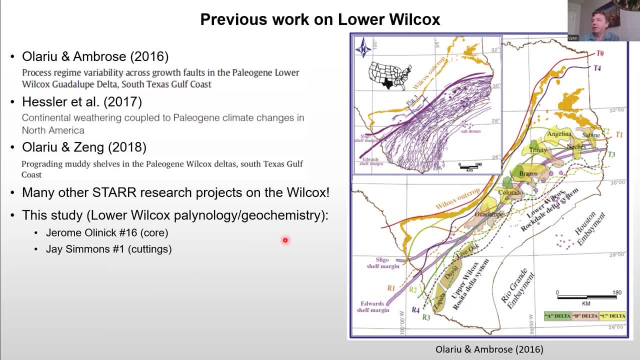 to the south And then it goes south east. So just to briefly mention a few, we have Alario and Ambrose looking at growth faults in the Guadalupe Delta. Angela Hessler has done work on continental weathering. Alario and Zing looking at deltas in the South Texas. 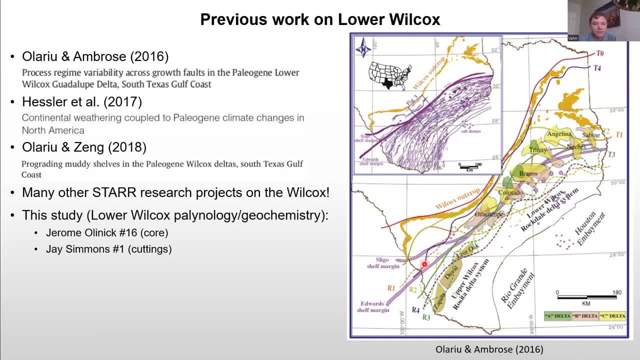 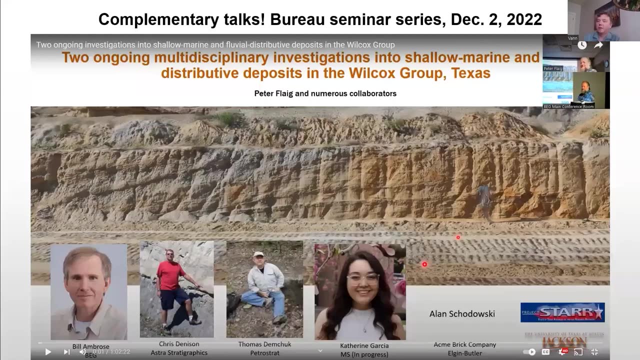 coast And there's a lot of other star research projects. This study is going to focus on the delta system, a core and cutting samples from the Jeremy Olenek and Jay Simmons number one. I also wanted to briefly mention the previous talk that you guys had at December 2nd. 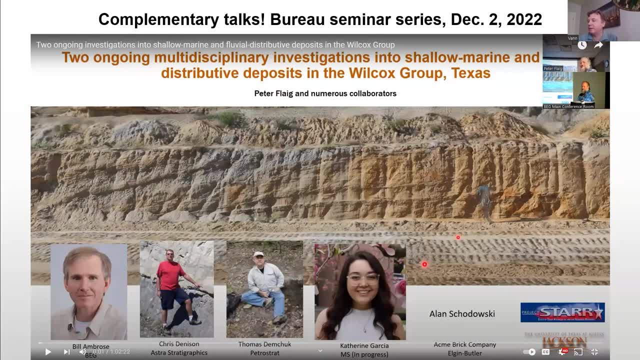 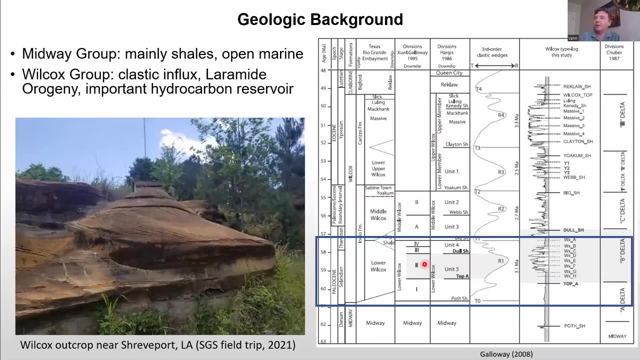 which would be a great thing to look at. you know, in addition to this, covering sort of different angles of this and looking at a bit of the younger Wilcox, the PETM section, So to give a bit of geologic background, 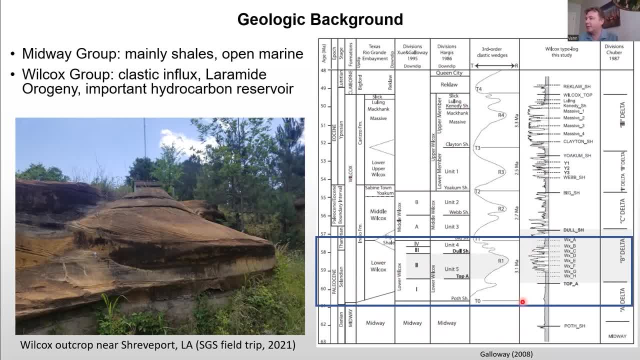 this is a Cenozoic, starting with Cenozoic in Texas. So after the end Cretaceous, you have deposition of this midway group which is mainly shales and open rain, And then you get a big influx of plastic material. 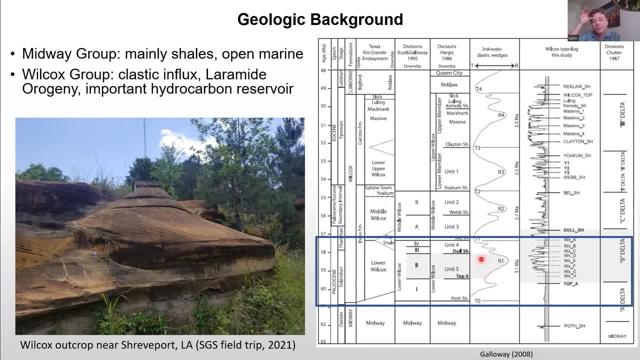 related to the Laramiterogeny and depositing some very thick sandstones and yeah And it that means it's an important hydrocarbon reservoir as all as well, And this is a outcrop of the Wilcox from Shreveport. 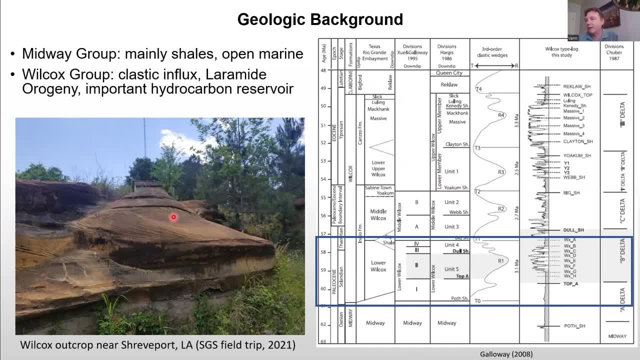 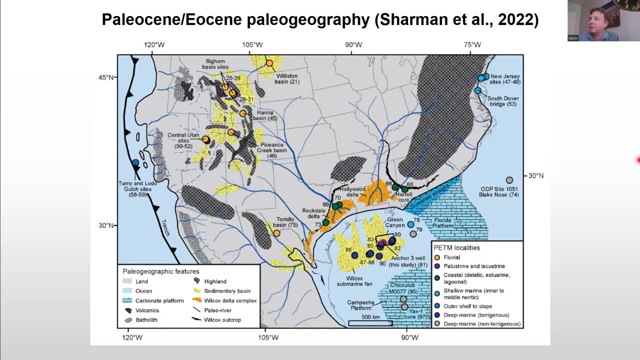 that I saw back in 2021. And you can see some of the. I'm including this map just to give you guys a general idea of what the paleogeography looked like around the time of the deposition of the Wilcox group. So we have some of these deep water systems here. 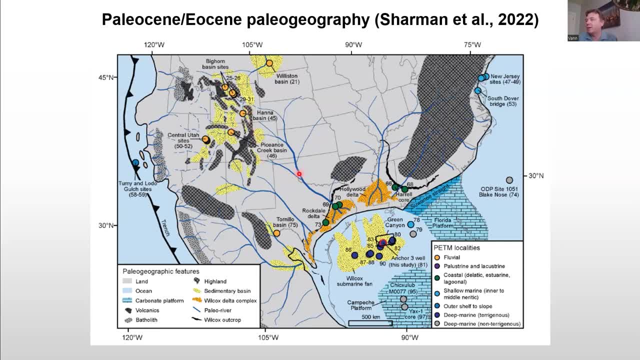 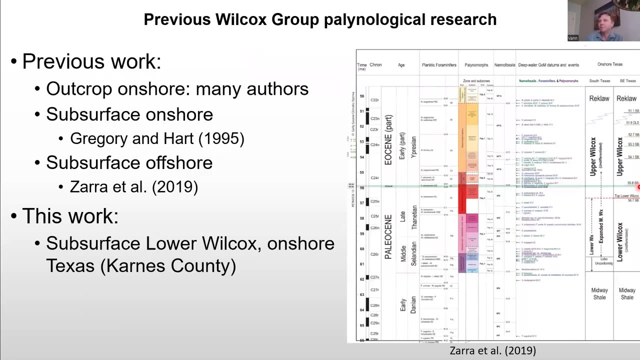 and then Delta system, all suspended Laramiter up here. This is also showing some PETM localities and I'll briefly mention Cretaceous was on looking at the PETM section and this Chicxulub core. So previous work I'd like to bring you over to take a look at some of the water systems. 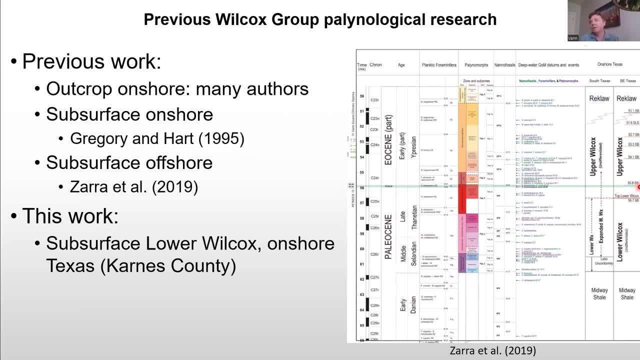 So this is a Cenozoic- the Langone water system here work in palynology in the Wilcox group. As far as outcrops onshore, a lot of people have published things going back to the 1960s. 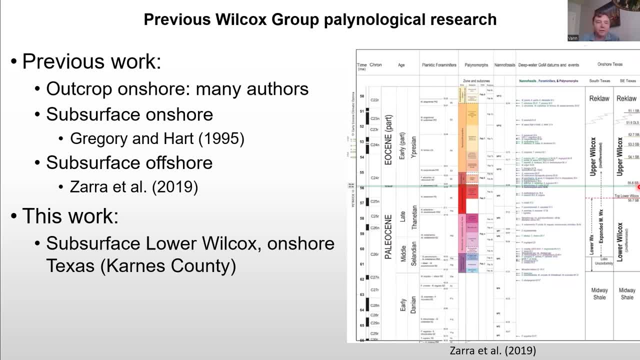 For the offshore subsurface there's a paper by Gregory and Hart in 1995, looking at subsurface Wilcox from Louisiana, And more recently there's a paper on the offshore subsurface by Zahra et al 2019,. 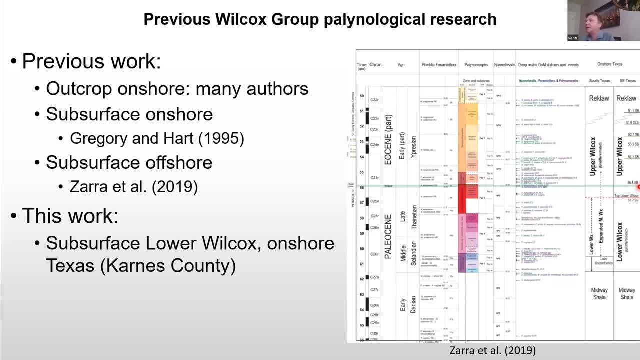 with Rebecca Horsworth. She was there and did a really good job coming up with a fire stratigraphic zonation for the Wilcox people And this work is going to be looking at the subsurface lower Wilcox onshore Texas in Carnes County. 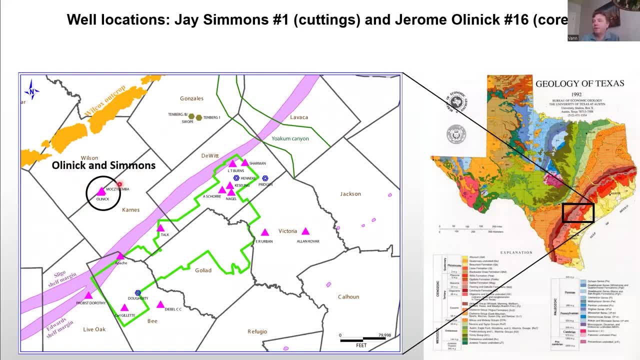 These are the locations of the well, the two wells here. They're right next to each other in Carnes County And this is just showing, really, our super-large well. We're both on a geologic mountain in Texas. We can sort of see the outcrops getting older. 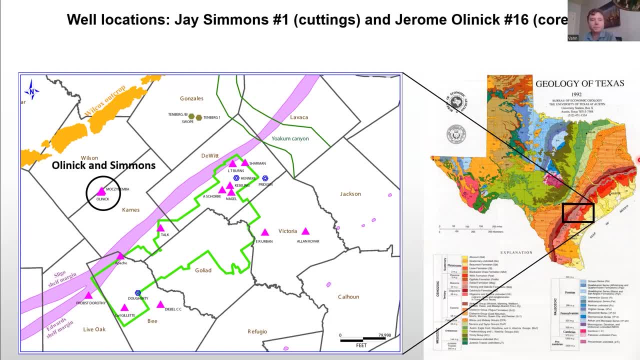 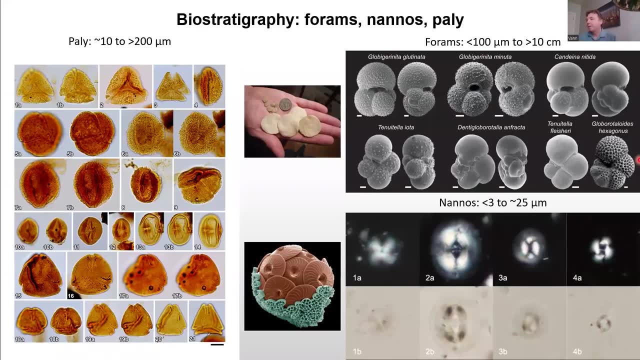 as you go northwest, paralleling the coast. So let's talk about the palynology And in case you're not familiar with these groups, I'm gonna go give sort of a short background. So these are examples of different types of call-in. 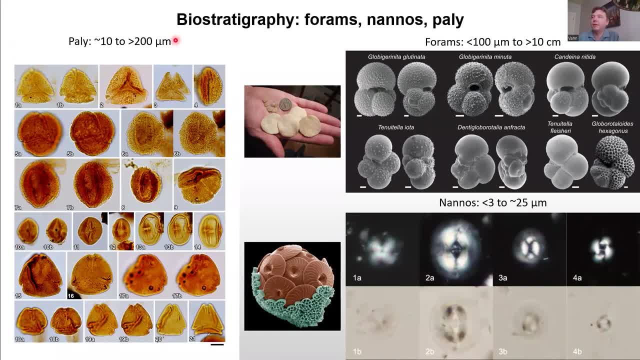 that we're seeing in the lower Wilcox. The size range here is for palynology in the Cenozoic is generally 10 to 200 microns, some rarely bigger than that. Can we have the other fossils Yeah? 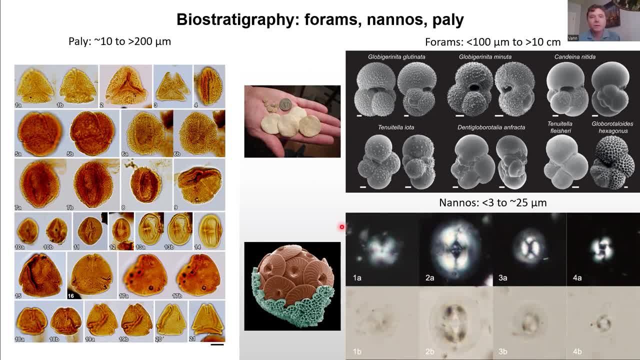 Sorry to interrupt. Can you get closer to the microphone? I think when you turn your face to the right we lose a little bit of sound. Oh sure, Sorry about that. Yeah, Thank you, Let me get the screen a little closer. 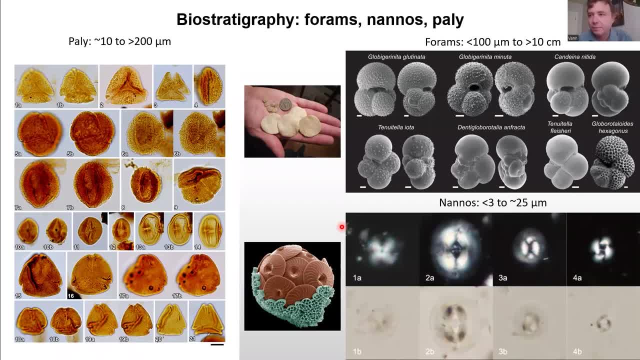 Is this better? That's good. When you do that, it's good. Yeah, OK, Cool Yeah. And so nanos are smaller than palynomorphs. They're also calcareous And forams, the kind that we look at in biostratigraphy. 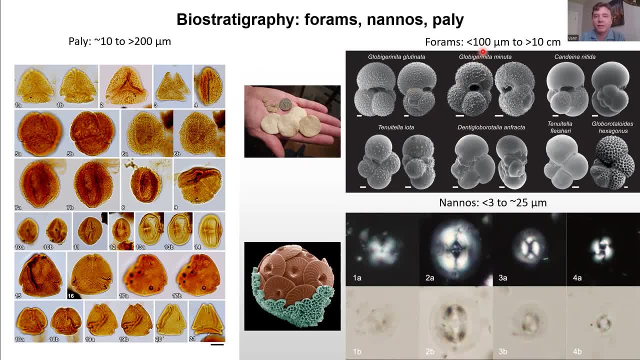 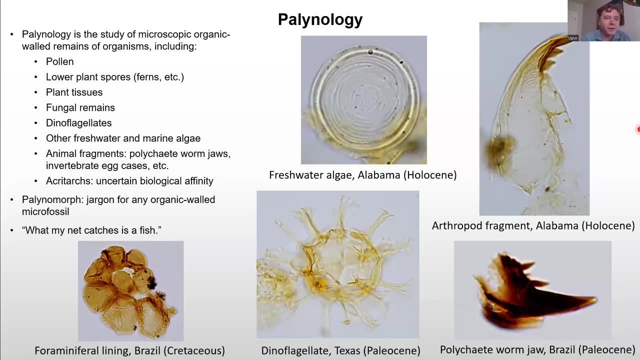 anyway are calcareous And they range from less than 100 microns to over 10 centimeters. In some cases they can get huge. These are individual single cell organisms, here bigger than a quarter. So what exactly is palynology? 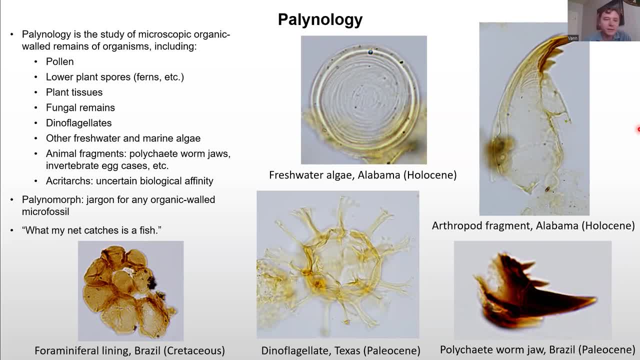 Most people think pollen immediately, and that's very important, But we also study lower plant spores, plant tissues, fungal remains, dinoflagellates, algae, animal fragments, aquitarchs, And we just lump those together and use a term called. 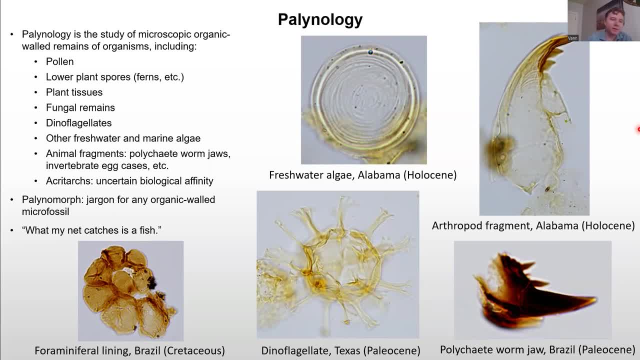 palynomorph, which just means any organic walled microfossil, And people have traversed this described it as what my net catches is a fish. So anything we see in the palynological preparations is fair game for palynology. 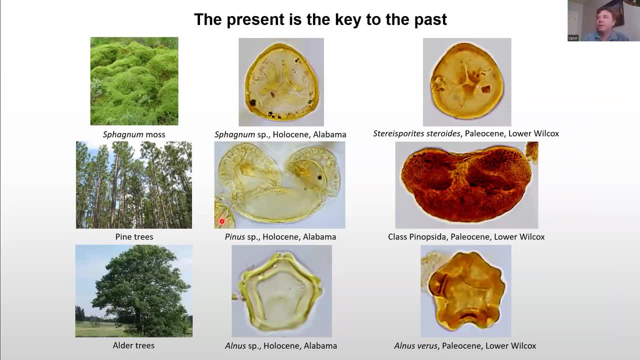 And an important thing to consider in palynology is that we want to figure out the biological affinities of these fossils and not just stamp collecting. We want to figure out what they're telling us about the paleoenvironment. So here's some modern pollen types and lower plant spore. 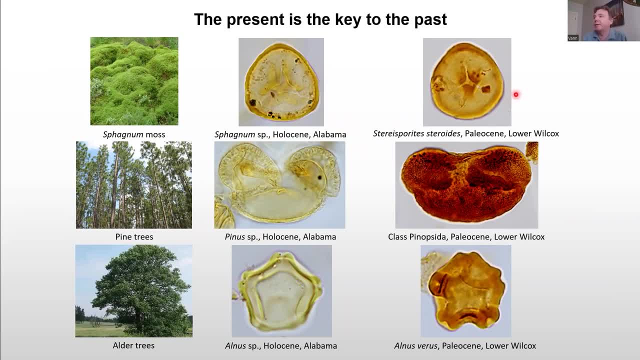 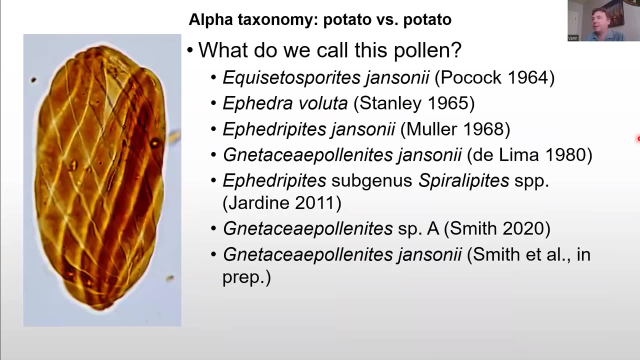 type from my Holocene research and then comparing it to similar types from the lower Wilcox. So you can see that we have sphagnum, pine trees and alder trees here And the pollen looks similar. And when I mentioned alpha taxonomy- 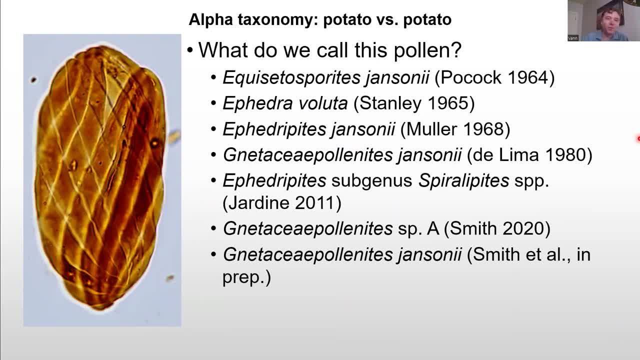 I just wanted to give this example. So what do we call this pollen? There's been a bunch of different names applied to this species, And people have had arguments about whether some of these are synonymous, And so part of what I'm doing is going through the naming of it. 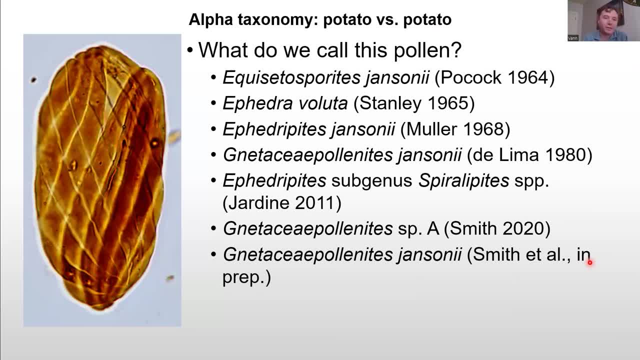 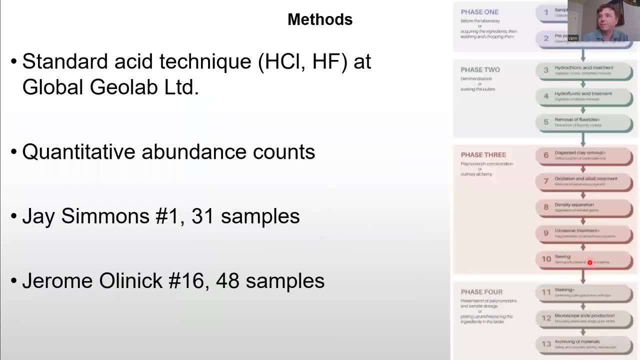 this and if it's potato or pothata, right. So the methods: we use the standard acid technique, using hydrochloric acid and hydrochloric acid to process the samples and put them on microscope slides for me to look at. This is done at Global Geolab in Canada. 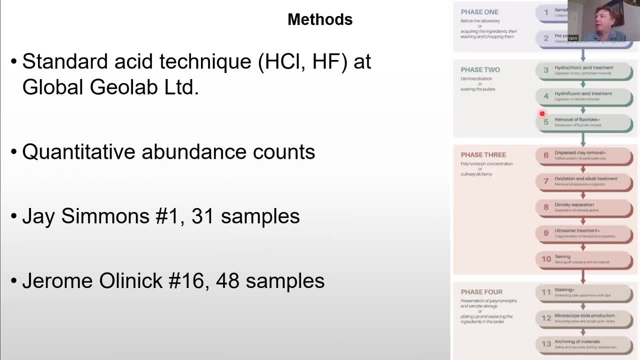 And I won't go into detail here. but the idea is you want to get rid of the carbonates and silicates And you're just left with the organic fraction, And I did quantitative abundance counts here. I won't go into detail about the methodology there. 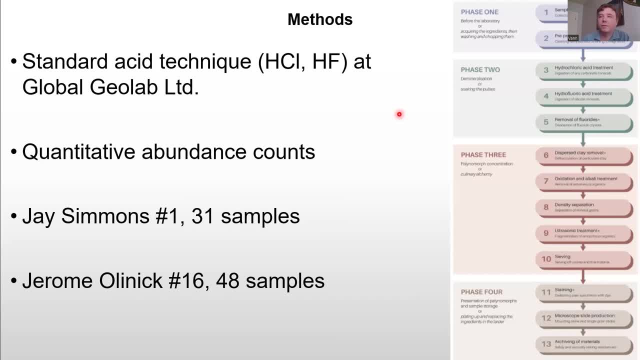 but I can if people have questions. So the samples that I have so far are 31 samples from the Jay Simmons and 48 samples from the Jeremy Olitik, number 16.. And we're going to be getting more samples, But analysis has been completed for palynology for these wells. 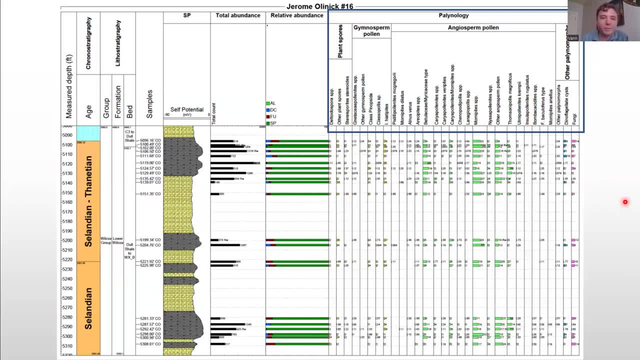 So this is the kind of output you get in strata bugs when you graph all of these pollen types. I've simplified the taxonomy here a little bit and grouping things together into genera instead of every species, Otherwise this would be unreadable. There'd be like 100 different types. 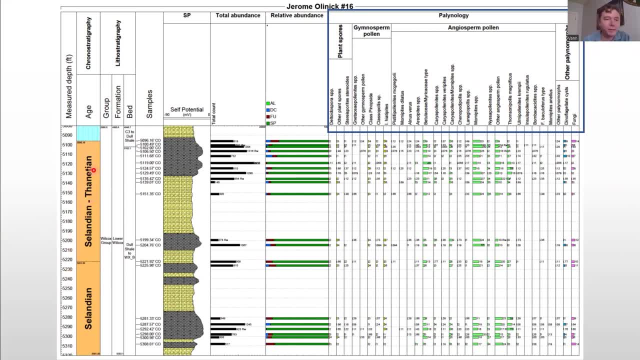 So this is the biostrata graph. I started graphic interpretation based on palynology sample depths, self-potential. This is total palynomorph abundance And then this shows the relative abundance of different types. So the dark green here is terrestrial pollen and plant. 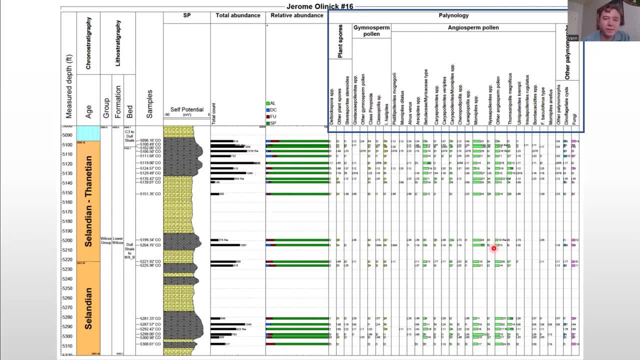 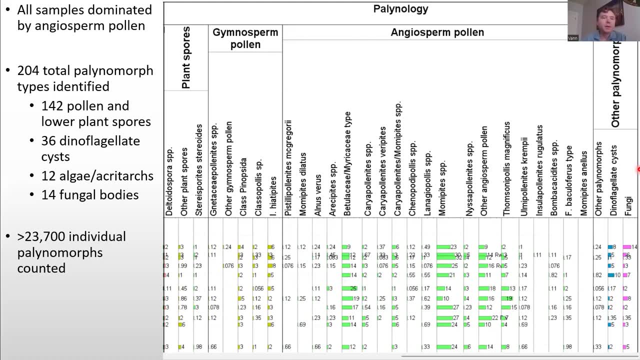 spores. The blue is dinoflagellate cysts And you can see that they're all mainly terrestrial pollen and plant spores that have been transported. So all the samples are dominated by angiogenesis. So we've identified angiosperm pollen. 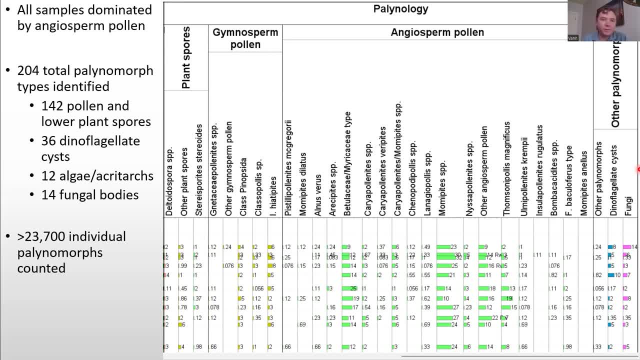 We've identified 204 total types, 142 pollen and lower plant spores, 36 dinoflagellate cysts, 12 algae, 14 fungal bodies, And these will all be described. This is well over 23,000 individual palynomorphs. 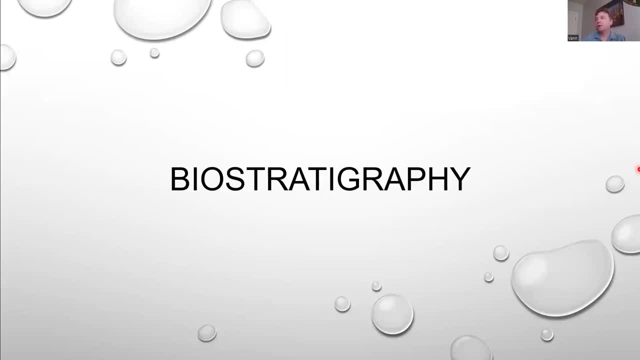 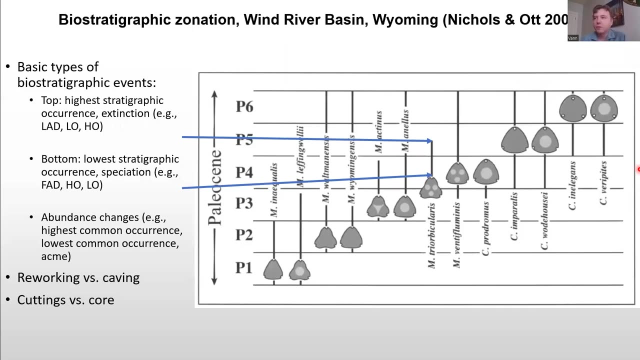 counted for these two wells. So let's talk about the biostratigraphy a bit. There's two very common types of biostratigraphic events. would be your top and your bottom. So this is showing this pollen group, Omypides, cardiopolinites, in Wyoming. 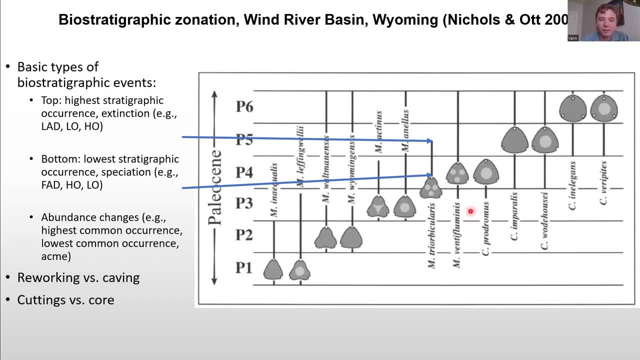 and using this as biostratigraphic zonation to split up the Paleocene. This one species, Triurbicularis, has a very short range, So when I say bottom, I just mean the lowest stratigraphic occurrence. Top, I mean the top. 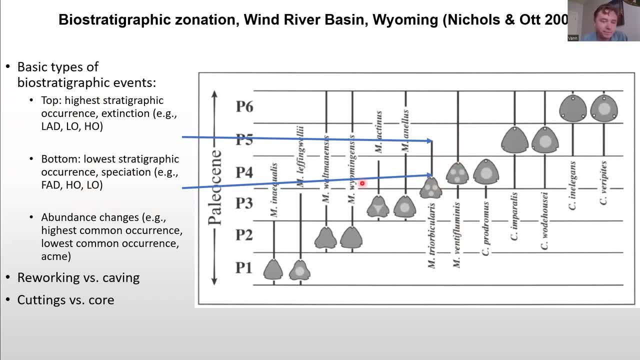 And people have different terms for this. I like using top and bottom, And then there's also abundance. changes can be events here, like the highest common occurrence, And I won't get into more detail here. We do have to consider reworking and caving in biostratigraphy. 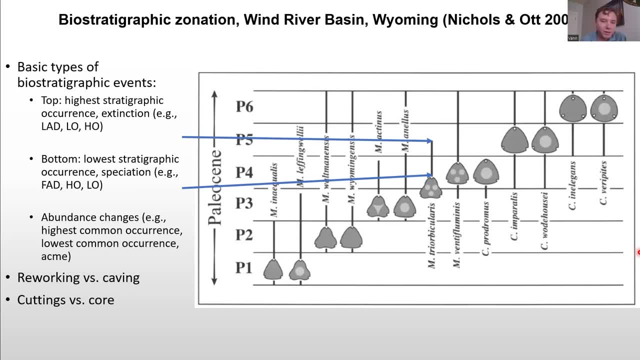 So reworking is when a pollen gets eroded and redeposited, So you might- if you don't know it's reworked, you might think you're older than you actually are, Sort of like a dinosaur fossil ending up in the Paleocene. 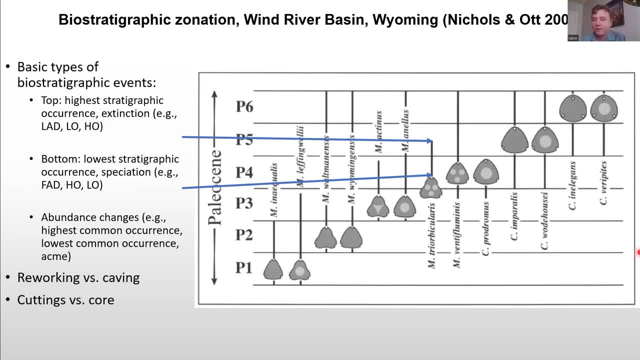 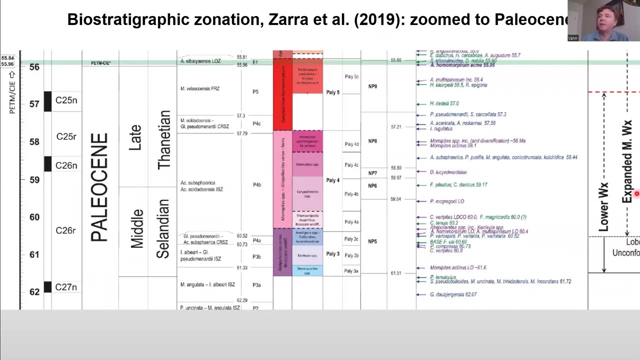 Caving is sort of the opposite problem that you have with well cuttings, where younger fossils can fall down into lower samples, And we'll go back to this zonation in a bit, But this is sort of zoomed in to the zonation. 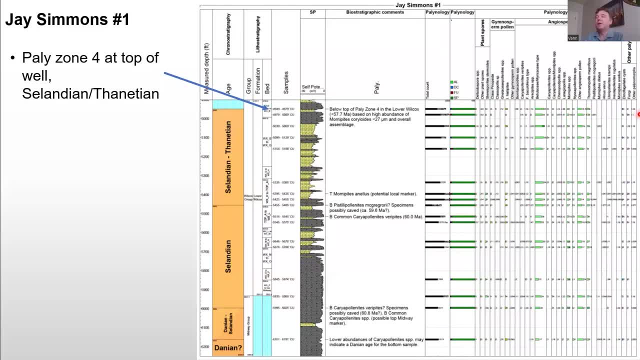 that Zahra has. that I'm basing this biostratigraphy on. So looking at J Simmons, number one at the top of the well, it is either Salandian or Phoenician. We're in Pali, zone four. There's this local marker that isn't in Zahra. 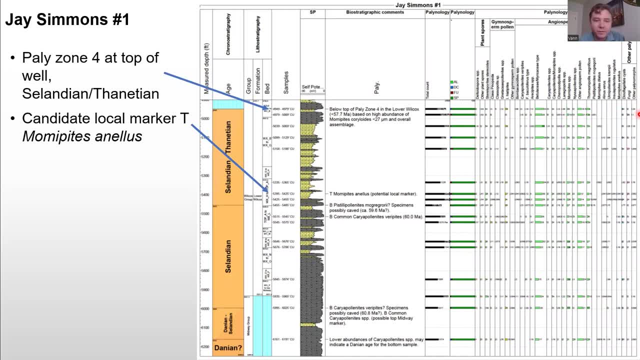 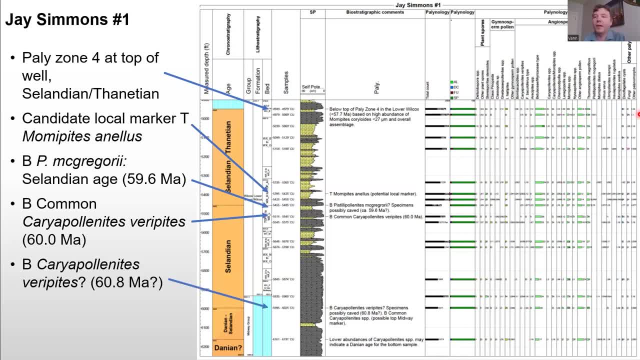 Then the base of common Cariopala 90s ripides And then the base of Cariopala 90s ripides, which is a little uncertain because these are cutting samples and they could be cave And it's possibly a top Danian at the bottom sample. 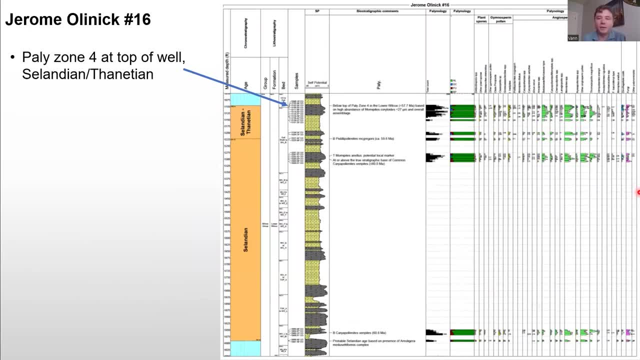 And it's possibly a top Danian at the bottom sample. Looking at the Germain-Olynyk, number 16, again Pali, zone four at the top, The base of P MacGregorii. The base of P MacGregorii. 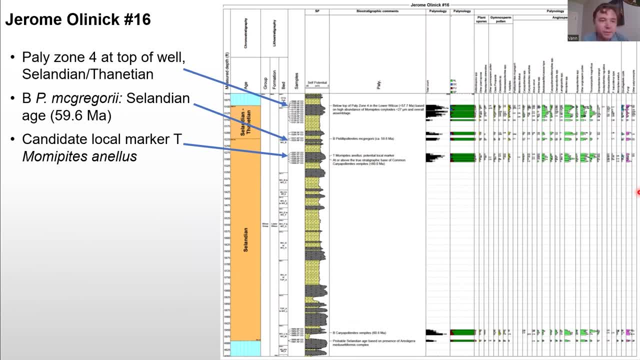 Again Pali zone four at the top. Again Pali zone four at the top. Again, that's local marker Moumypides annulus. These events are quite close to each other and they're actually flipped in stratigraphic order. 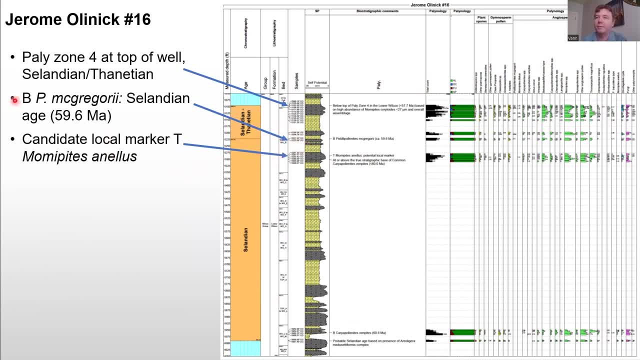 So they're pretty close in age And analysis of borwells will help clarify which one is truly above the other. We again have base common Cariopala 90s ripides. There's a big sample gap here due to poor palentomorph. 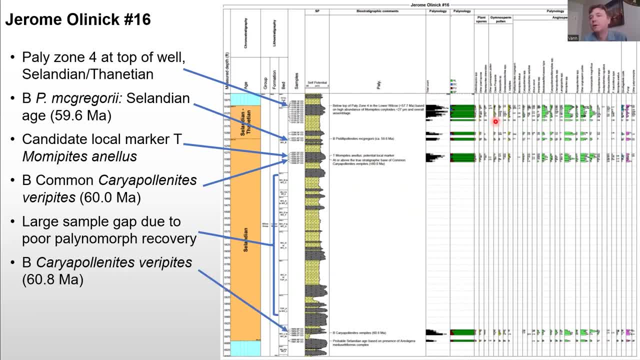 expected poor palentomorph recovery and sands, And then Bayes' cardiopoly 90s baryphetes And the bottom sample we think is Stelcelandia NNH, based on the dinoflagellate areolaegera meducetiformis complex, And we 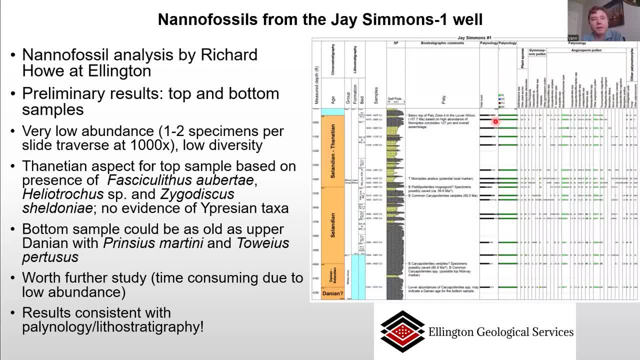 recently have some initial results from the some nanofossil analysis of the J Simmons. well, by Richard Howard Ellington We these are very preliminary. He's just looked at the top and bottom samples of the J Simmons. well, so far, And in those slides it's very. 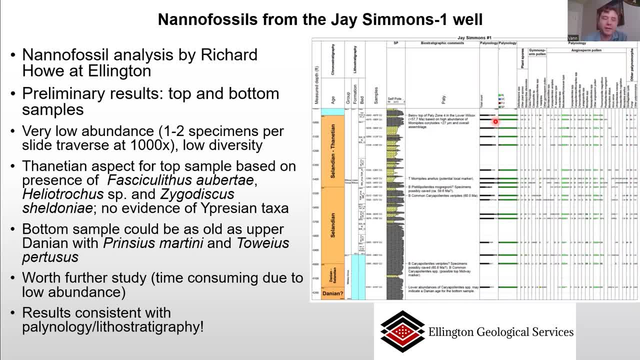 low abundance: one to two specimens per slide traverse at a thousand times magnification, And it's low diversity Which sort of can make it more difficult to get a more precise biostratigraphic age on it. There's a aspect for the top sample based on the presence of these species and no evidence of Epresian. 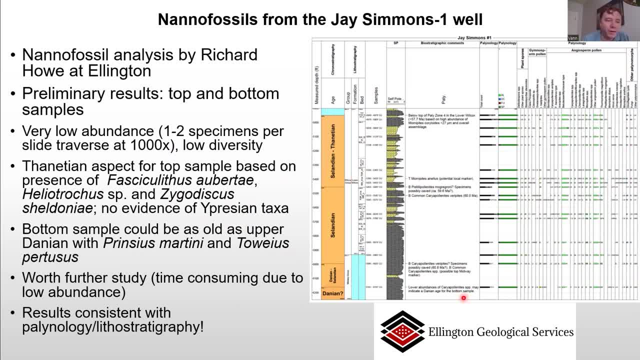 or early Eocene taxa, And the bottom sample could be as old as Upper Danian, with Prenzius martini and Tueus protusus. This is definitely worth further study. It is probably going to be quite time-consuming if the other samples are as rare as this one, but it's nice to 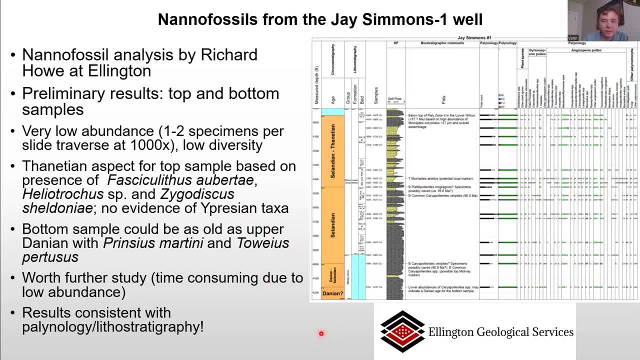 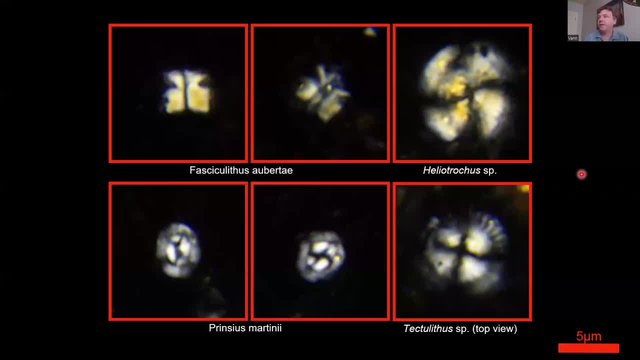 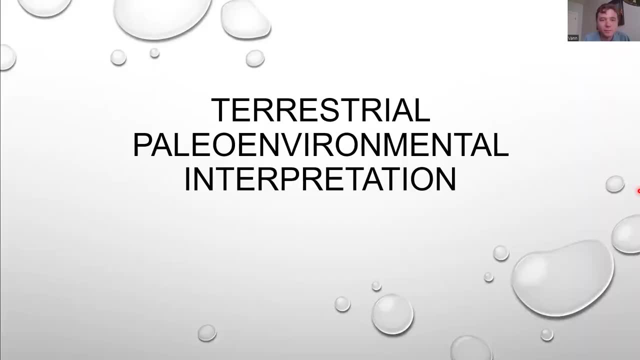 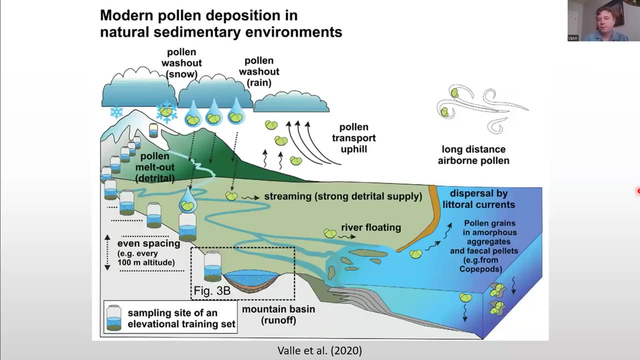 see that the initial results are consistent with the palynology and lithostratigraphy. And just to show you what these nanos look like, here's a couple of pictures of them from the lower Wilcox. Okay, let's talk about the paleoenvironmental interpretation. This is a nice cartoon by 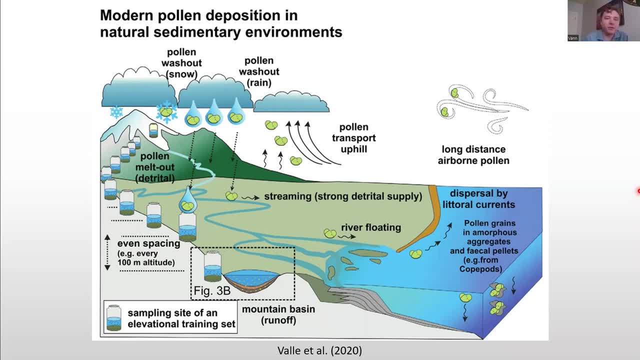 Valli et al 2020. Showing what happens to pollen after it leaves the plant. So pollen can be transported by wind and water. It can end up in rain and snow. So the pollen that we're seeing in this shallow marine area is a mix of local and long-distance transport and fluvial transport. 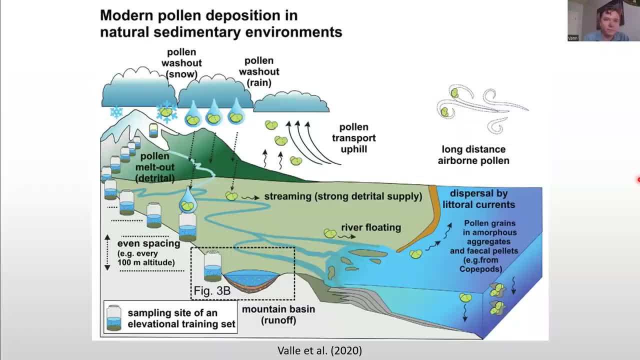 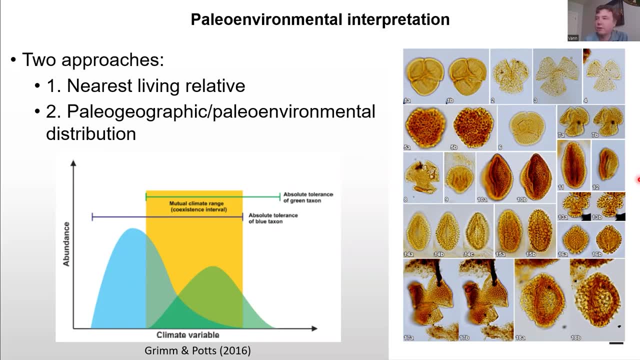 and wind transport. So for the paleoenvironmental interpretation of these pollen and plant spores, there's two approaches. The first is nearest living relative. So what is you look at? you figure out. what is this pollen, what affinity does it have? what family or modern genus is it? 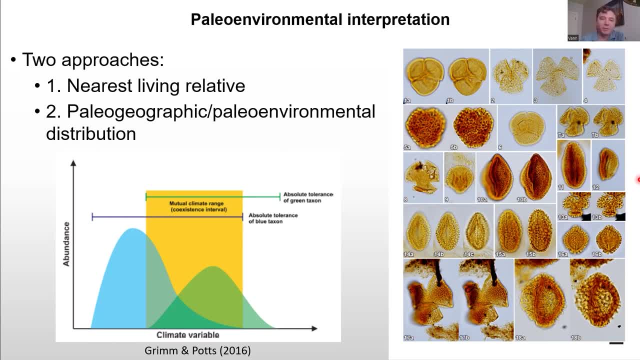 and what environments do they live in? today? This becomes more uncertain the older you get back in time. And then there's also the paleogeographic and paleoenvironmental distribution. So if you are looking in the Cretaceous and you see a pollen type, and you only see it in the 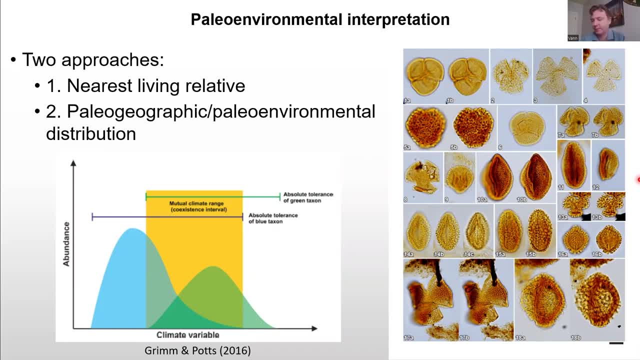 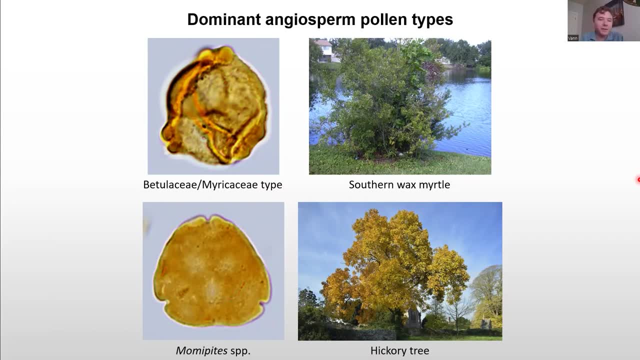 paleotropics, then it's, you know, indicating tropical conditions, that kind of thing, And so I wanted to show you some pictures of the pollen types that I'm seeing and also pictures of modern plants that we think are pretty similar to what 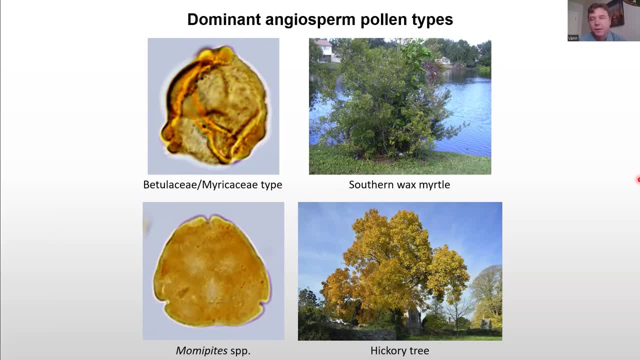 the plants look like that produce these pollen in the Paleocene. So a very common type is what we call this Betulacea myracaceae type, which includes several genera, but it might have looked something like the southern wax myrtle with similar 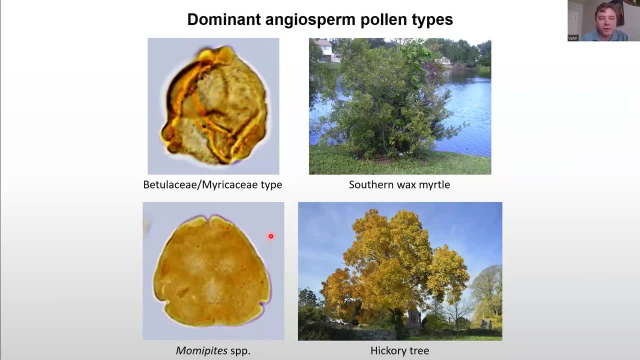 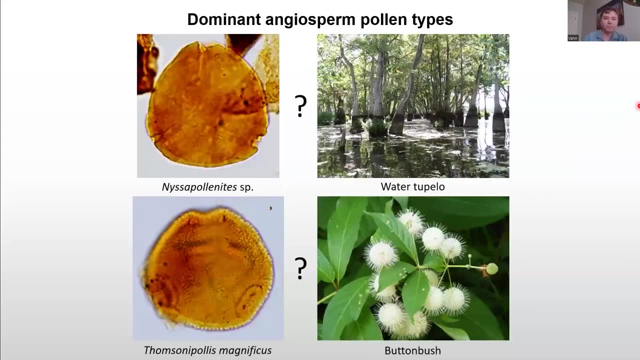 environmental preferences. Monympodes and karyopolinites are very common and they're related to hickory trees, Some of the other more common pollen types. The affinity is less certain, So Nyssa pollinites. despite the name Nyssa, it is somewhat uncertain, but it may be related. 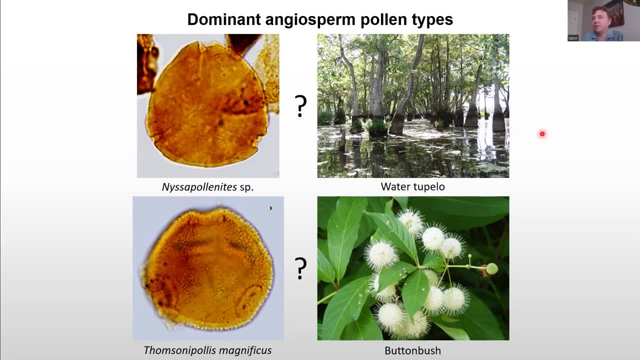 to modern water-tooth blow, which is sort of a lowland forest marshy type tree, Thompsonopolis magnificus. this is probably even more uncertain, but it is quite common. Maybe a relationship with the rubyaceae? This is a buttonbush from Texas. 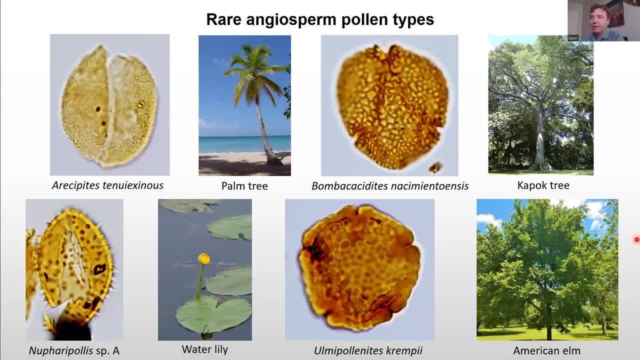 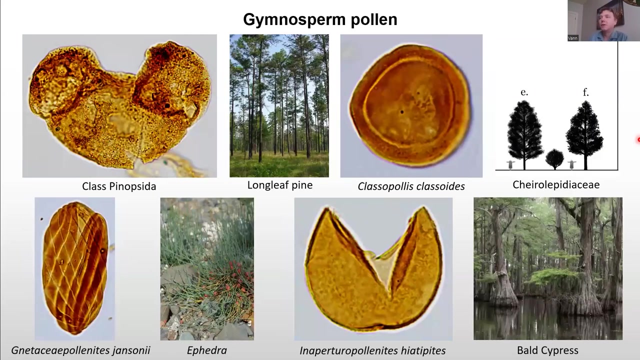 Some of the less common types. We have palm tree pollen, pollen of this tropical tree, Kapok tree, similar to it, Pollen from water lilies and elm tree pollen. Then, for the gymnosperm pollen, we have some pine pollen. 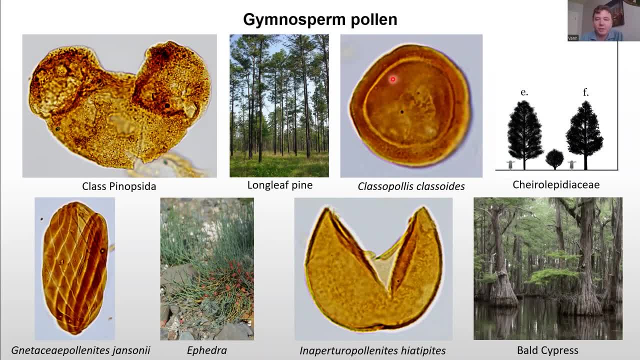 We have this distinct group called Clasipolis that I'll talk about in a bit, Pollen related to modern ephedra, which generally lives in arid conditions, and pollen that may represent something similar to bald cypress, although some other groups can produce it. 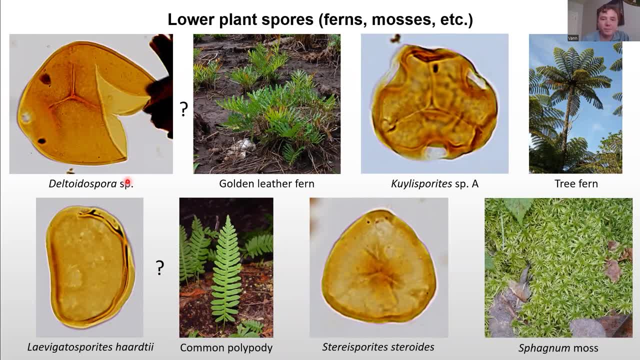 For the lower plant spores. these are the more common types, well, except for this one. I included this one because it's interesting. You can be pretty confident that this is a tree fern pollen, Cyathea Deltoidospora. could be from a lot of things, but maybe it looks something like this: golden. 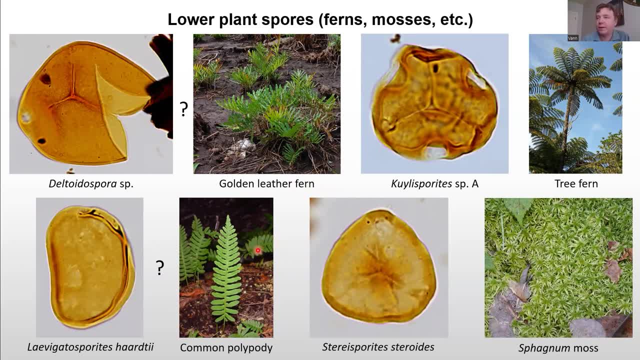 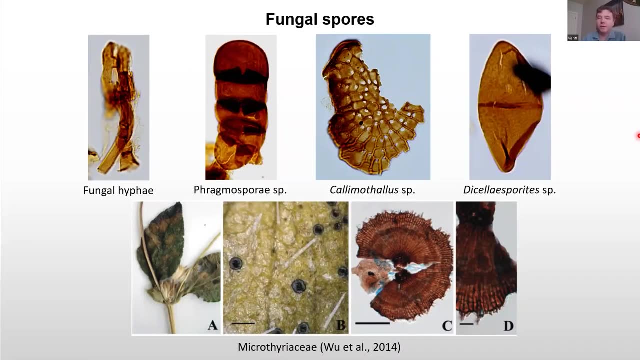 leather fern, Lavagattosporides, maybe another fern, something like this common polypodi- And then Sterosporides. steroides is basically sphagnum, which generally indicates moist conditions. I've also identified the fungal Spores here. 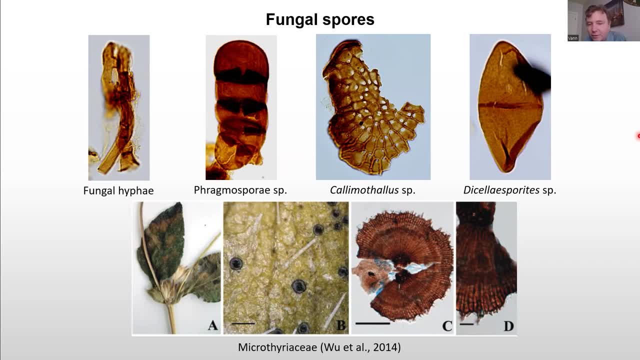 They're generally not as biostratigraphically useful as the pollen, plant spores and dinoflagellates, but that might be partially due to the fact that people haven't really studied this as much as the other groups, And so there's a lot of sort of types who are not too sure about the lower biological affinity. 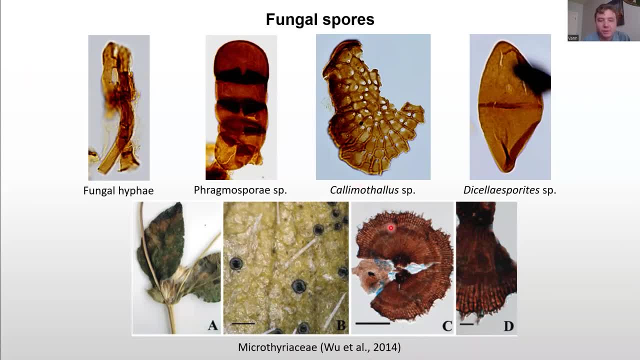 But there were some interesting types that I'm pretty sure are microtheory ACA. These live on plant leaves and sort of eat decaying plant leaves. So you can see modern ones here, And this is the lower Wilcox version. We're also seeing freshwater algae. 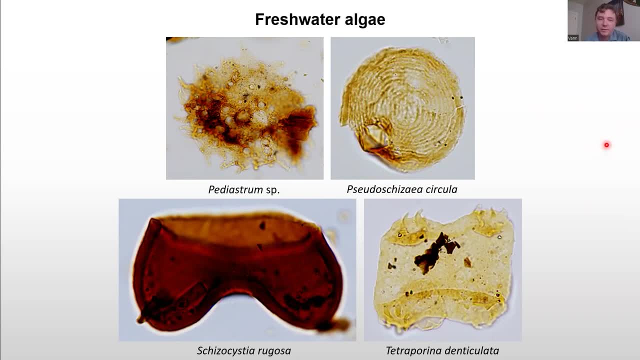 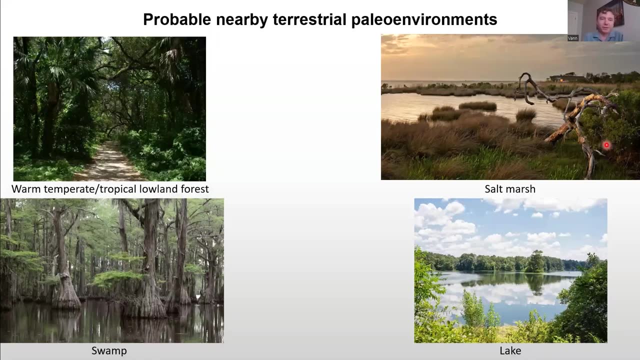 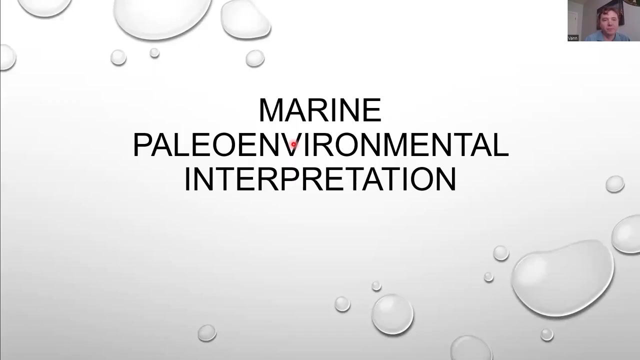 And most of these freshwater algae types are related to the modern algae family Zygna metaceae. So that's a lot of pictures, But the sort of big picture is that they generally indicate probable nearby terrestrial paleoenvironments, A lot of them indicating either like a warm temperate to tropical lowland, forest, swamp, salt, marsh and lake environments. 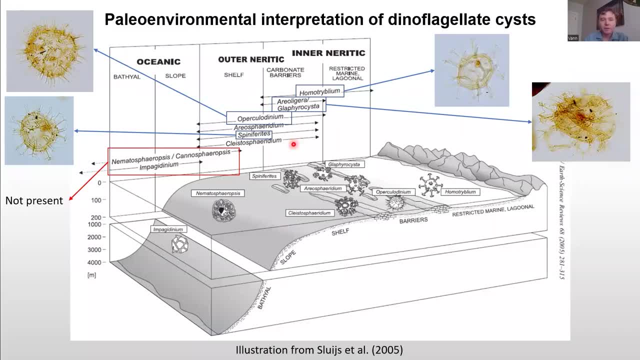 So the marine paleoenvironmental interpretation. The dinoflagellates are not as common as the pollen plant, They're not as common as the pollen plant spores And often they weren't very diverse, not as well preserved, And the most common type was this Aperculidinium type. here 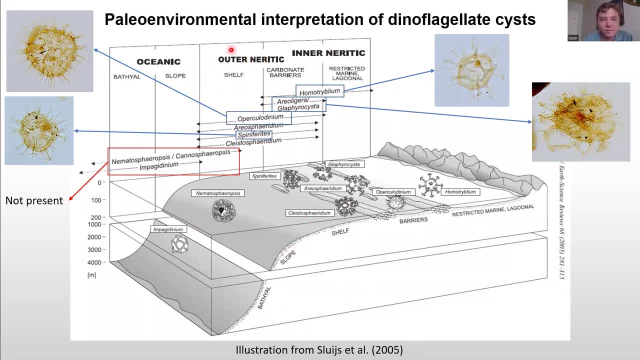 And this is an illustration from Slough et al 2005.. So these blue arrows and boxes indicate that we're seeing them in the core. So we're seeing genera that indicate neuritic conditions. So we're seeing genera that indicate neuritic conditions. 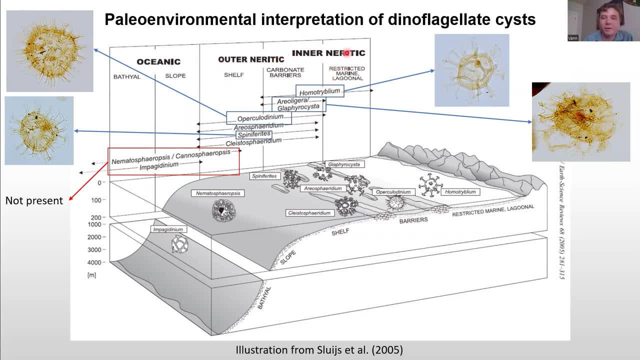 So we're seeing genera that indicate neuritic conditions, And some of them may be even restricted marine, And some of them may be even restricted marine, And what we're not seeing are these groups that are more oceanic. So the assemblage is indicating shallow water. 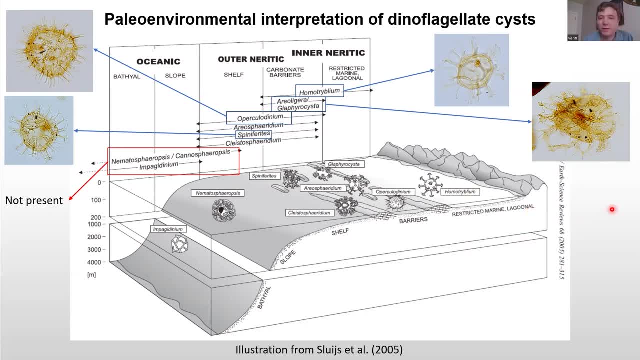 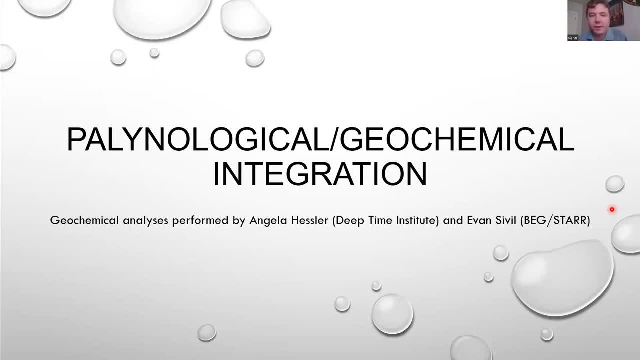 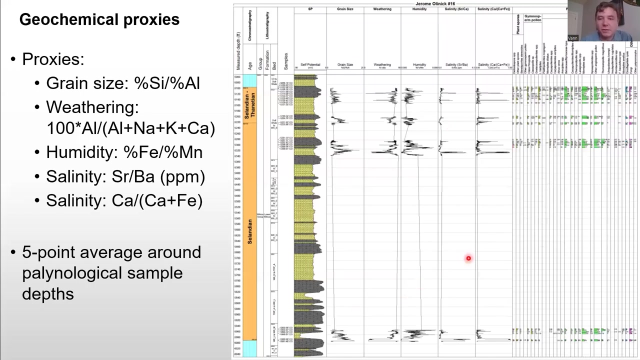 And also probably normal marine salinity most of the time. And then the next thing I'll talk about is the geochemical integration, And these analyses were performed by Angela Hessler at DTI and Evan Civil at BEG-STAR. This shows the PALI data together with the geochemical data. 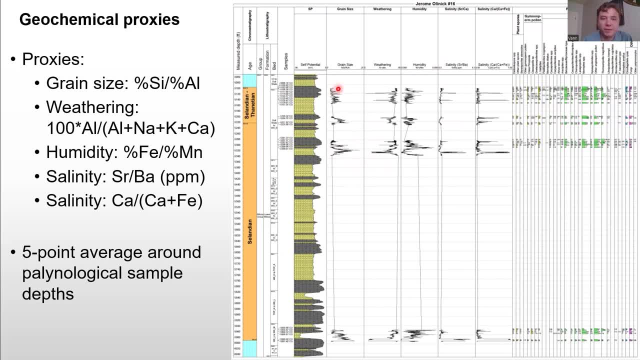 The geochemical data is very high resolution sampling. as you can see, There are various proxies that we have that I won't go into detail with, like grain size, weathering humidity. There are various proxies that we have that I won't go into detail with: like grain size, weathering humidity. 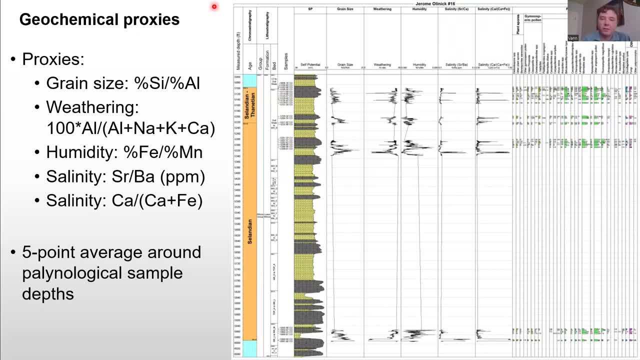 Two salinity proxies. So I wanted to compare that with some of the relative abundance data to see if there was a correlation. So we took a five-point average around the PALI logical sample depths and then just compared the values to see if there was correlation. 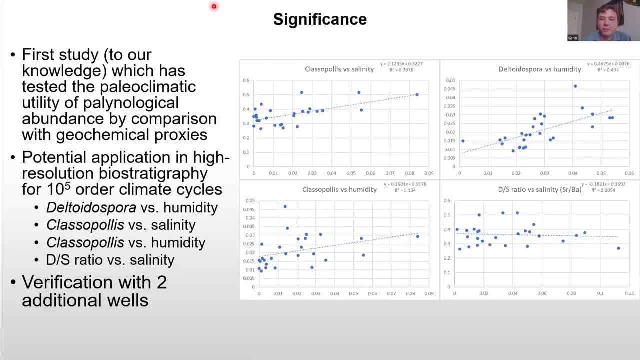 So this shows some of the correlations between the PALI and the general waterdress, the PALI and the GeoChem. To our knowledge, this is the first study which has tested the paleoclimatic utility of palynological abundance data by comparison with geochemical proxies. 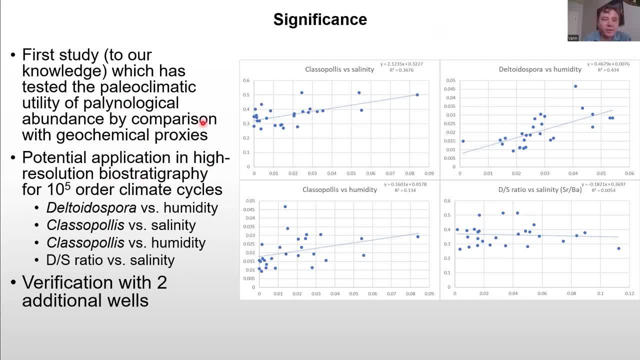 And it has a potential application in high-resolution biostratigraphy for like 10 to the 5th order climate cycles. Some of the groups that worked particularly well. deltoidospora versus humidity has a positive correlation. So, as expected, deltoidospora- 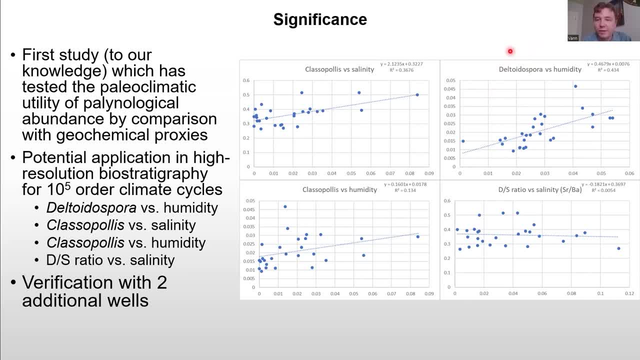 we think that it is more common in moist conditions. So the positive correlation is expected and pretty good. Classopolis versus salinity is also fairly good And this is an extinct group but it's thought to have lived in arid and are like salt marsh coastal. 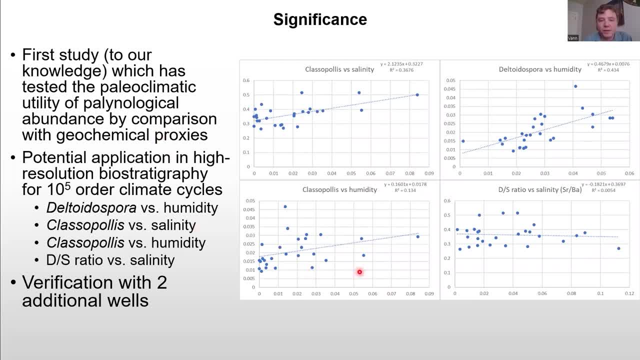 habitats. Looking at it versus humidity, it's actually not well correlated in the opposite direction, because we would expect it to be more common in more arid environments. So it sort of indicates classopolis is more of a salt marsh indicator than a ruta tea indicator. 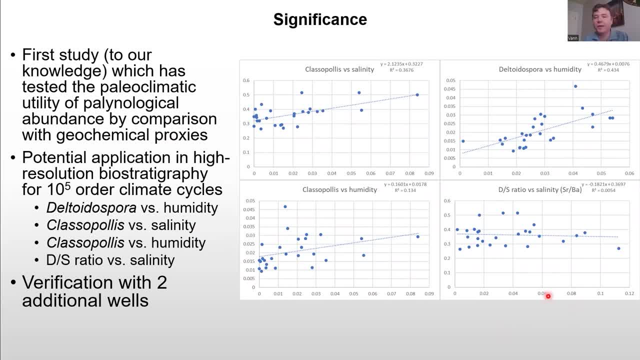 Look at the DS ratio. So this is the ratio between marine dinoflagellates and terrestrial pollen and spores. Generally, you expect if you see more dinoflagellates that you have more of a marine influence. but I'm not really seeing a relationship with salinity. So this 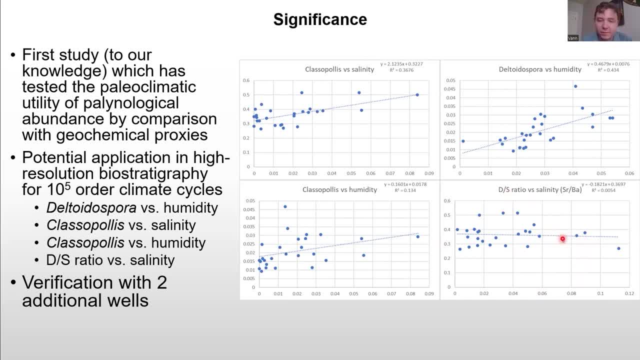 may be. it may be that the DS ratio is telling us more here about the amount of fluvial input than the salinity directly, And we're going to look at two additional wells, So we're going to do the same thing and see if we see the same trends here. So the conclusion: 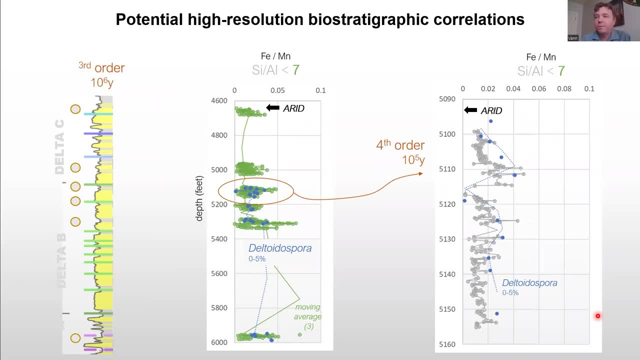 well, first there's a potential high resolution biostratigraphic correlations we could make and sort of climate cycles we could look at with the assistance of this relative abundance data. So we took deltoidospora and this is just showing a comparison. when you graph, 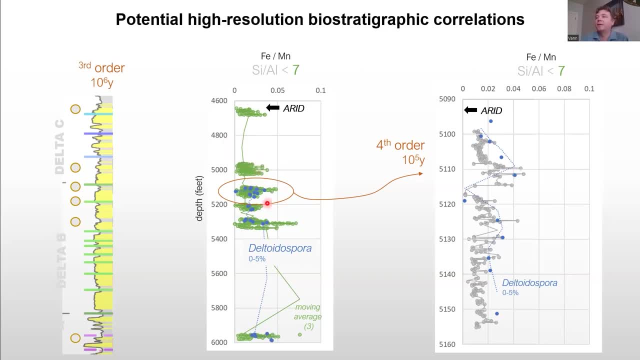 this aridity or humidity proxy with the deltoidospora abundance And you can see, if you look at this, the trends match up pretty well. This is zooming in on like 10 to the fifth order cycles here that are tracking together pretty well, which is encouraging. 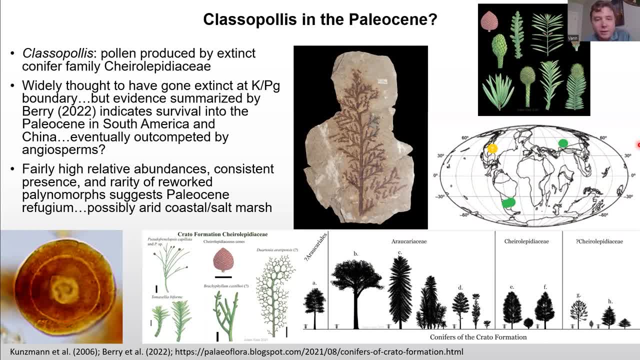 Another important thing to mention is this group, classipolis. So it's pollen produced by an extinct conifer family called the Cairo lepidaceae, And it's widely thought to have gone extinct at the end of the Cretaceous, along with the dinosaurs. But there's evidence. 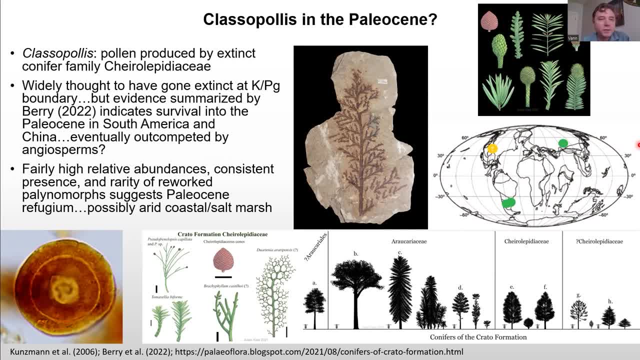 summarized by Barry in 2022, which indicates survival of the group into the Paleocene in South America and China, And he provided several possible explanations for their eventual extinction, possibly competition by angiosperms. And this is a map from Barry showing in green the locations. 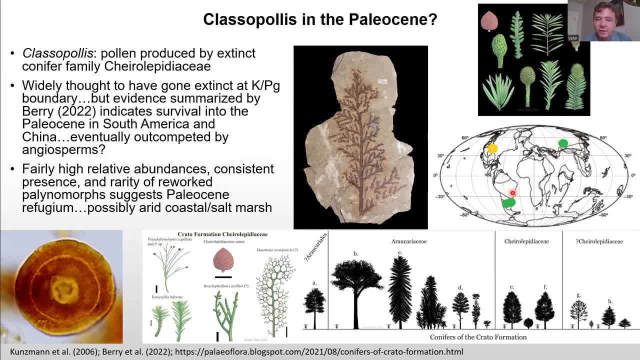 where he's confident that there's Paleocene occurrences of this group and then a question mark over North America, And so I think, in our course this is classipolis. by the way, we see fairly high relative abundances of this consistently present, and there's a rarity. 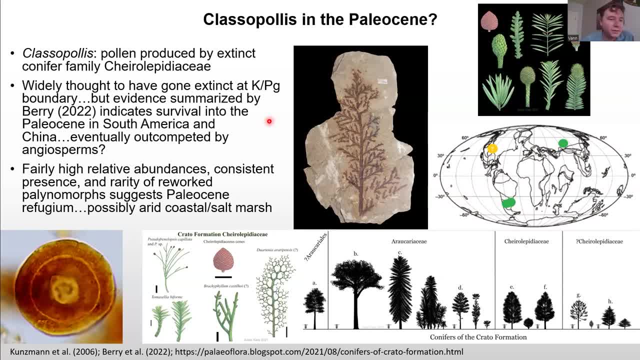 of other reworked pollen from the Cretaceous. This all suggests that the classipolis is in situ and is a Paleocene, And Barry also mentioned that these were sort of living in arid coastal salt marsh environments. So this is: we're interpreting this as a late refugium for this extinct conifer family. 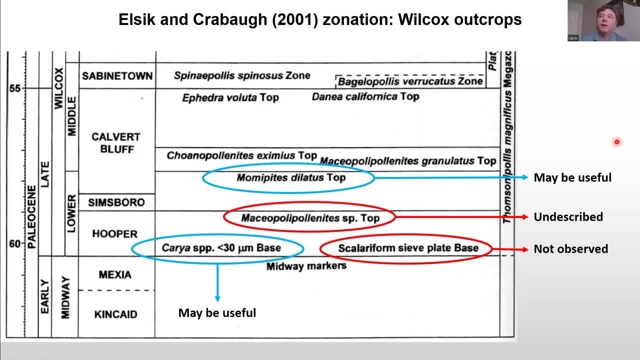 This is a comparison of our results with a zonation- an earlier zonation by Elsik and Kravah- from Wilcox outcrops, And so I'm just paying attention to the lower Wilcox here. So this type may be useful. 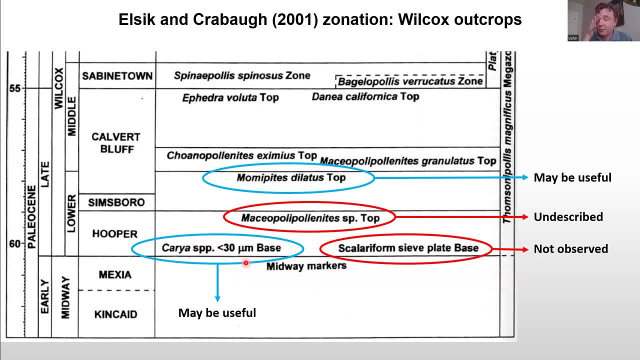 this Caria species less than 30 microns, Presumably. he's talking about Caria pollinates here, not the modern genus. I didn't observe any of these scleriform sieve plates, And this Maceo pola pollinates species is undescribed, so I can't really be certain what they mean. 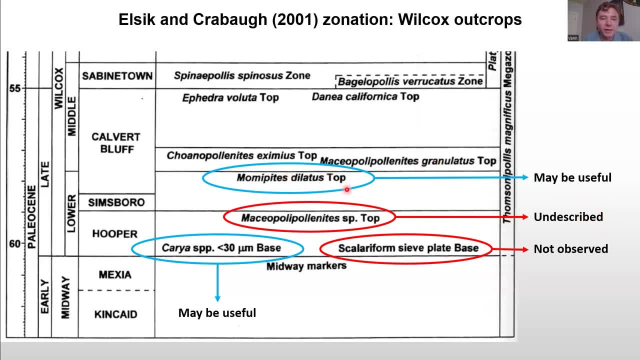 by that And Momyphetes dolatus. top also appears to be good because we're seeing it throughout our samples, and our samples are almost probably exclusively lower Wilcox with maybe a little bit of middle Wilcox and Danium at the top and bottom. 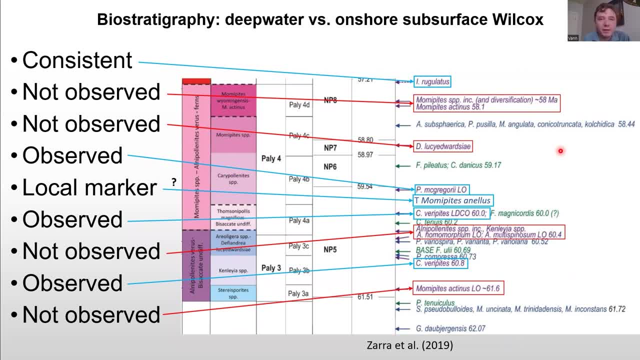 So let's compare it with the deepwater, the deepwater zonation by Zara. So some of these groups, the species over here that are not in boxes, are either nanofossils or forams. These are forams, these are nanofossils, so we're not looking at those, I'm just going. 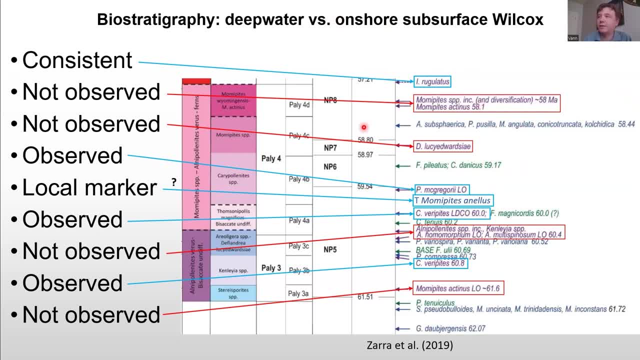 down through this column and seeing which of these events worked and which didn't. So at the top here, Encelopolinates rugulatus- we didn't actually see the top here, but it is consistent with what we've seen. We do see this species in the core, we just don't. 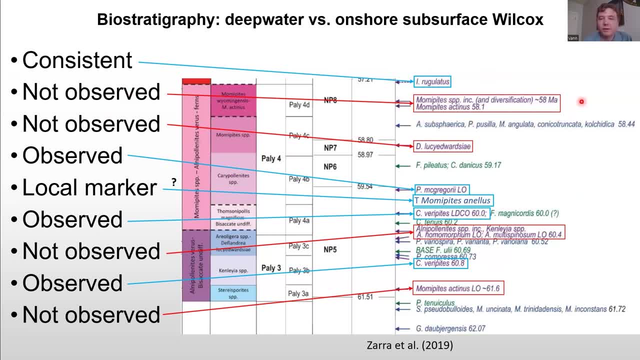 see the top. We didn't observe these abundance changes in Momyphetes clearly, and Momyphetes actinus appears to be absent. This may be because we're getting a more regional signal from these onshore cores and the deepwater. you're seeing a broader pollen source area and Momyphetes. 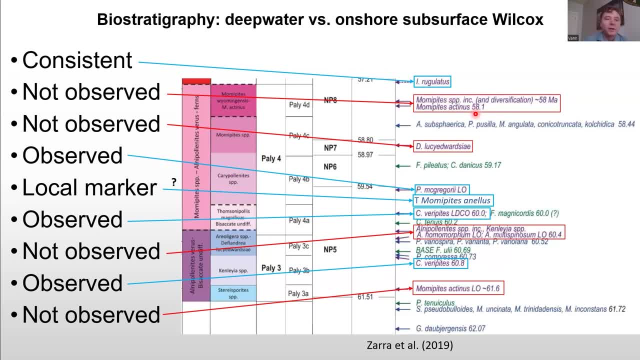 actinus is living elsewhere. We didn't observe this dinoflagellate species, but we did see some change in the quality of life. But our dinoflagellates were fairly rare and not super diverse, so that's not too surprising. 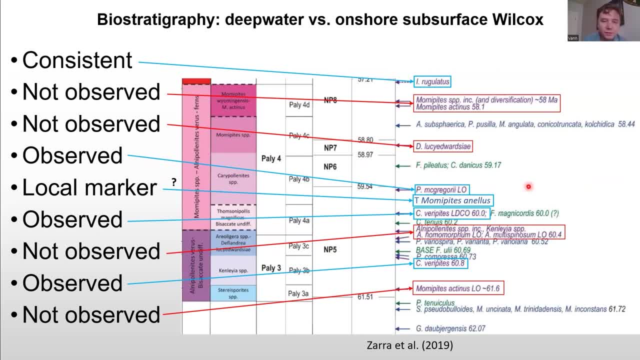 P mcgregorii was a very useful event. We have this local marker, T momyphetes annulus. that fits right in here, maybe a little bit above P mcgregorii. The next two wells should clarify this. 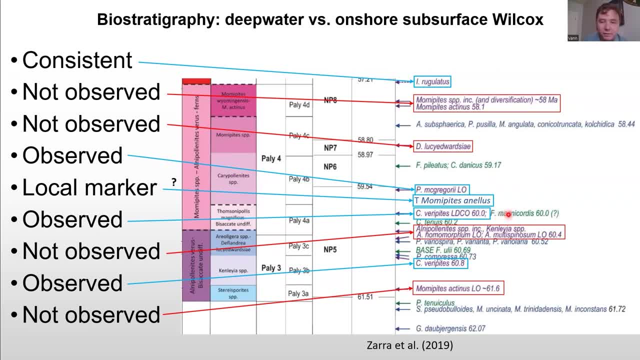 We see C viripides as a useful event. We didn't observe these abundance changes and we didn't observe these lowest occurrences of Apectiodinium comomorphum and Maltospinosum. Again, these are dinoflagellates, so it appears. 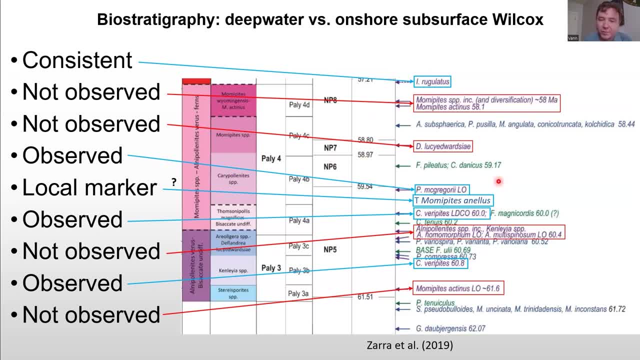 like the dinoflagellates, are not working quite as well. I only saw one specimen of Apectiodinium, and it wasn't one of these species in the core C, viripides. the bottom of this is a good event. 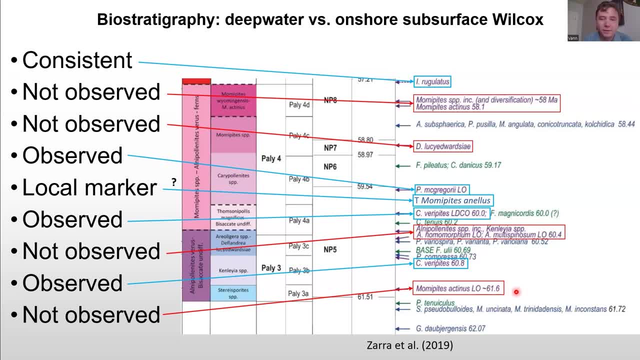 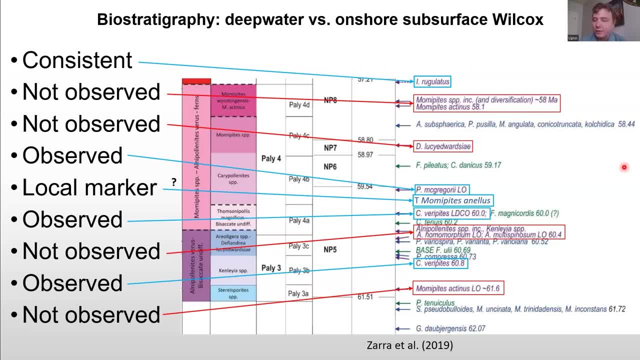 We have some interesting results from these two wells and I'm really excited to further work on this. We have more work to do with integrating this palynology with lithostratigraphy and the geochemistry, and we're going to be looking at two more wells, so stay tuned. 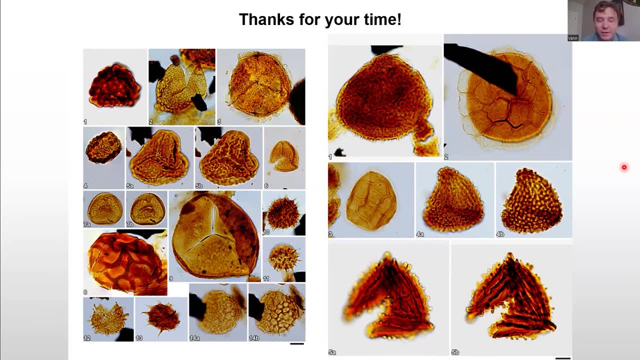 and the geochemistry- and we're going to be looking at two more wells, so stay tuned. and the geochemistry- and we're going to be looking at two more wells, so stay tuned. I want to say thanks for your time and I look forward to any questions you might have. 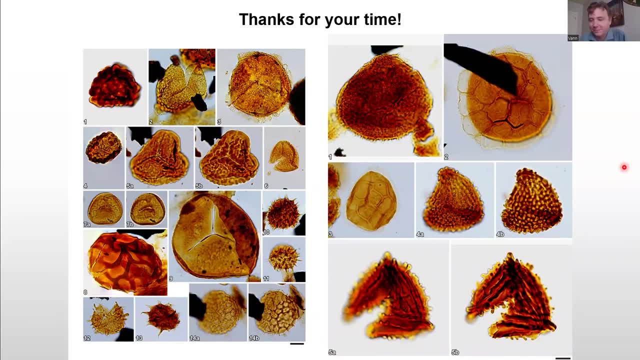 Thank you, Van. That was excellent. We're doing great on time and if there are any questions from the audience, please don't be shy. Any questions or comments? This is Rebecca Hackworth. I have just a comment for Van. 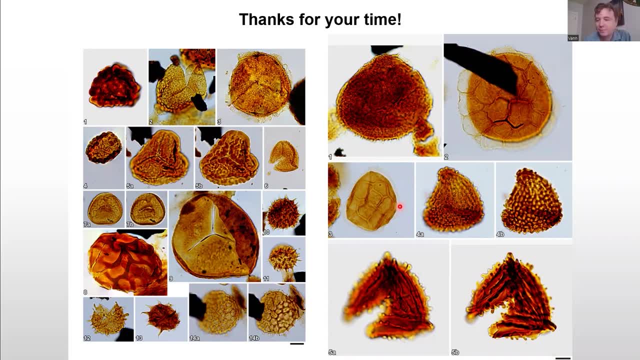 Sure, Hi Van. It doesn't surprise me at all that you're not seeing the actinus. When we get in the deep water I notice as we go different parts of the Gulf of Mexico. actinus is more prevalent, so there may be some localized actinus. 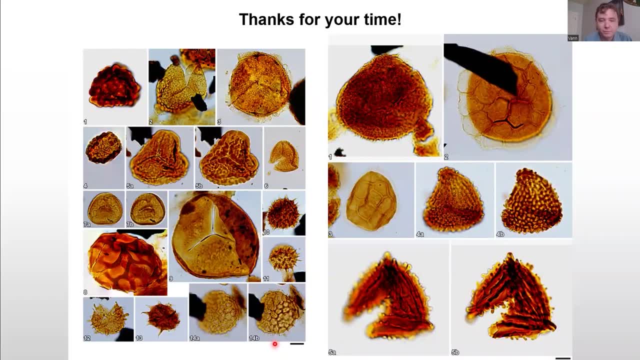 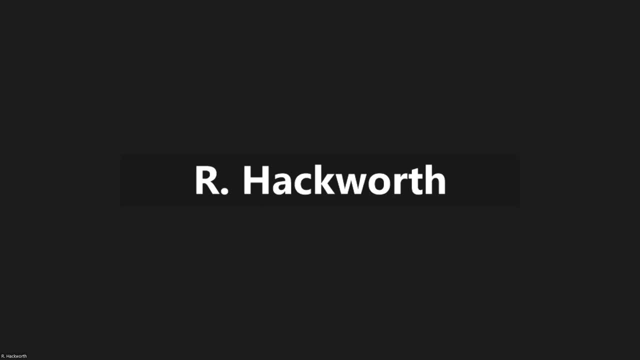 there may be some localized actinus, So you may not be seeing it. It would be interesting, if you get more on-shore course material, to find out what areas on shore you're seeing actinus versus where you're not seeing it. Cool, Yeah, well, I'm glad to hear that you're not too close to it. 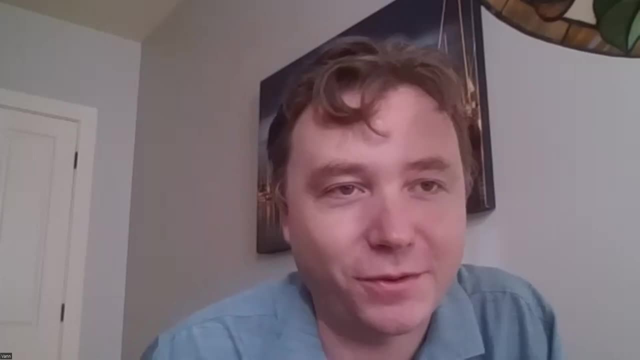 Thank you, Van. Yes, We'll be getting started. I'm just checking if it's already not Okay. Okay, All right, Okay, We're going to give you two minutes and then we'll continue. surprised by that absence, I was definitely on the lookout for that And the other two cores we have. 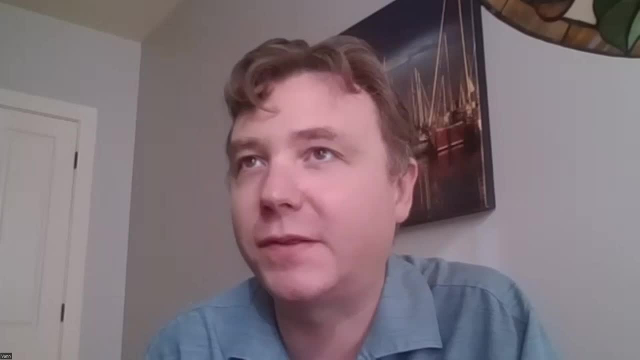 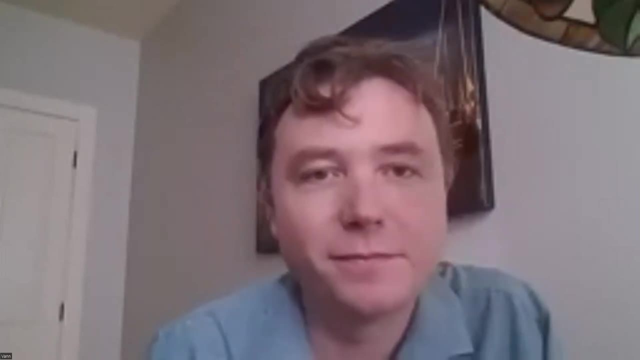 are not quite as close together as these, so it'll be interesting to see if that species pops up. Yeah, very much so. It's good that people are doing some onshore work in this section, because there's definitely not a lot of onshore work done A lot of times because that, you know, these intervals are cooked further. 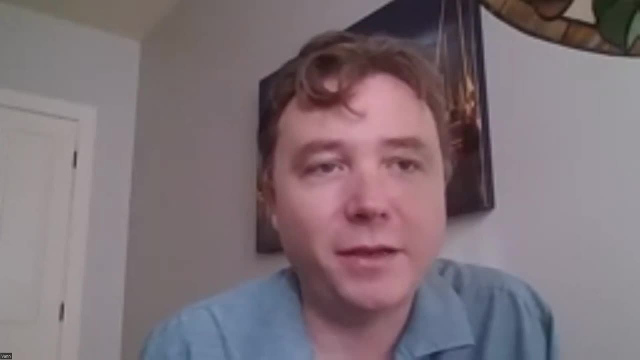 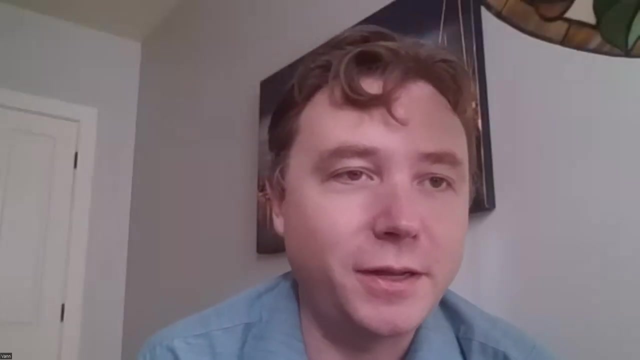 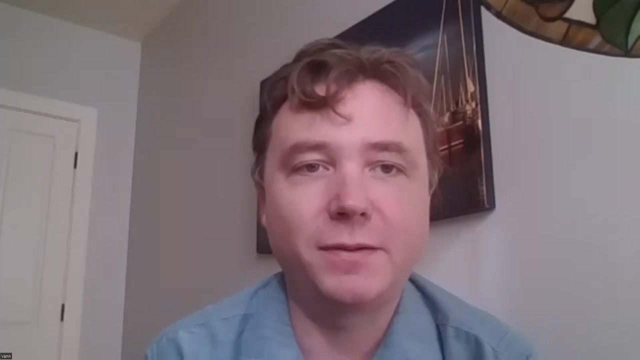 down dip in a lot of those cores, so I'm glad you got some good recovery. The recovery looks fantastic. Yeah, yeah, there is really good preservation and most pretty much all of the samples and abundance was good. Yeah, it worked well. Yeah, I think we were a little bit nervous. 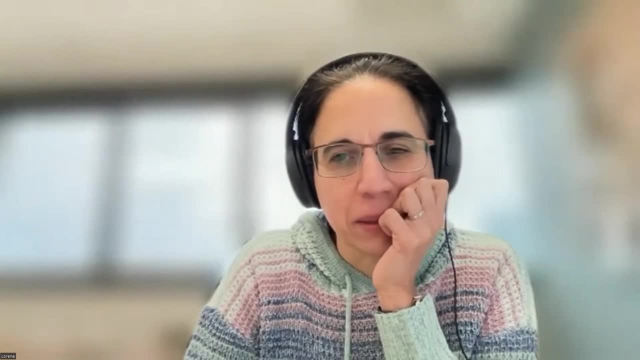 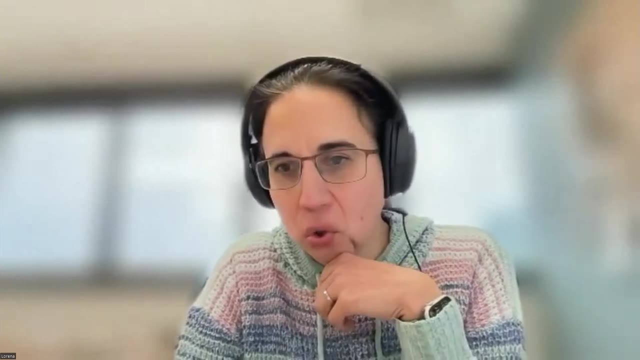 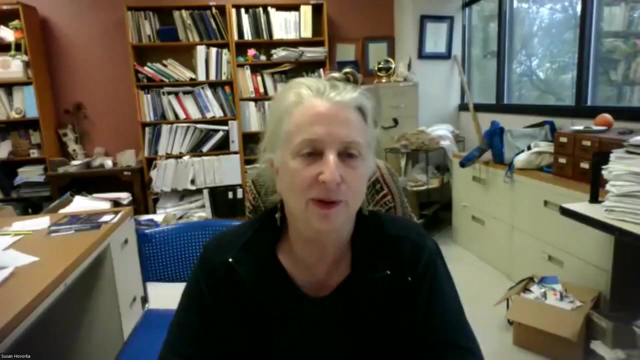 when we were collecting the, The samples first, but we have been surprised in a good way with the recovery. So I think thank you, Rebecca, for your question. I think Sue Havorka has a question. Sue, Hi, I enjoyed this talk very much, Van. Thank you very much. I'm not a Wilcox or a. 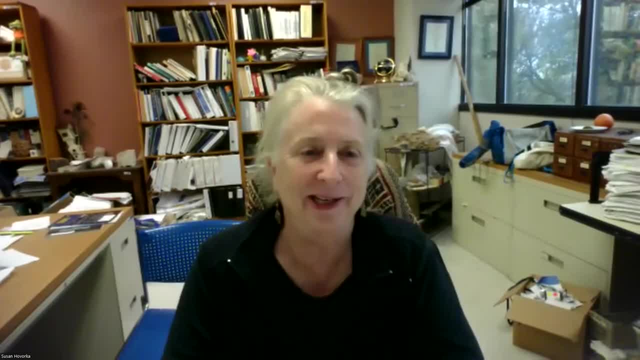 palynology expert, so it was really clear and illuminating for my purposes. I wanted to know about if you could talk about the, What the pollen, The palynology, tells you about, the changing, The changing environments, from sand-rich intervals to mud-rich intervals. Do you collect this out of? 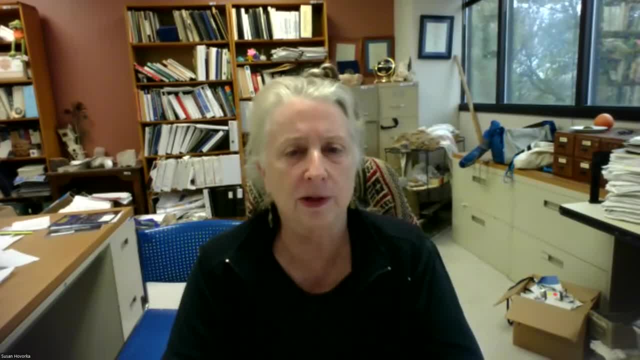 Where do you collect your samples? Out of the reservoir intervals or you have these also. I mean all the different muds from the inter fluvial kind of, you know- soils to marine incursion, you know, between delta marine incursions. So what's represented in your set? 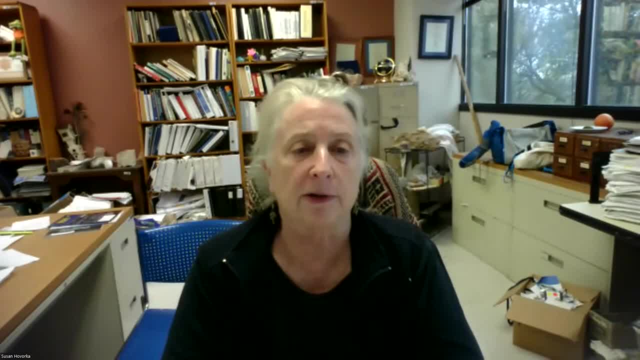 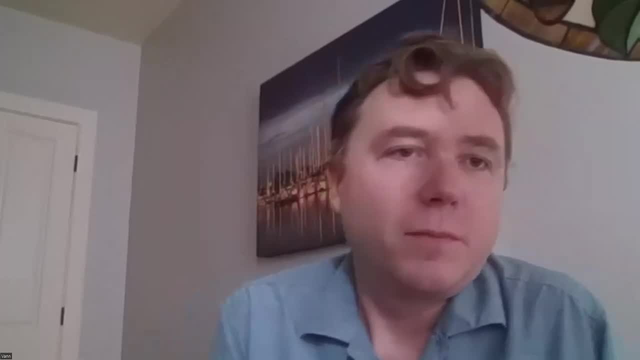 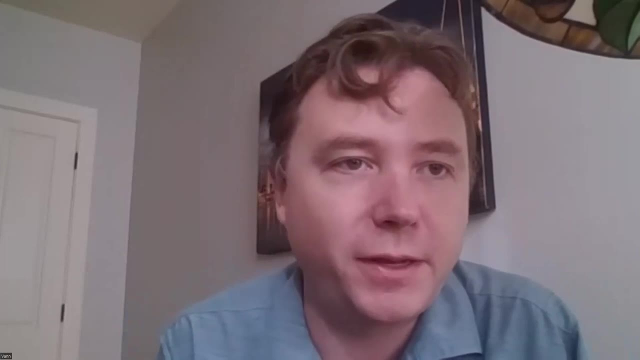 And can you reflect on. Especially, I'm interested in the environment of the finds, the mud, rocks, Yeah. so before I started on this project, Carlos Santos was associated with it and he did some of the sampling. He did the sampling of the core and picking the well cuttings to use. 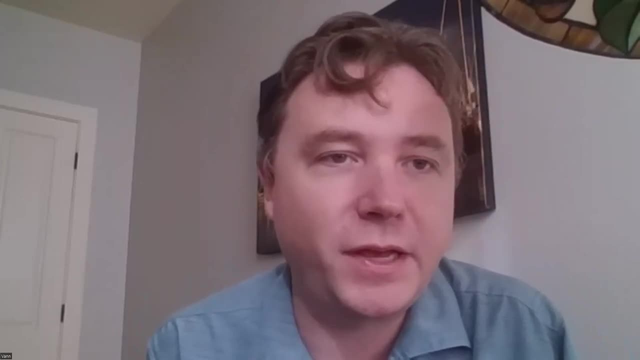 So we sort of avoided the The coarser sand intervals, because generally they don't have good preservation as well, Because sand continued to put more pressure on sand, you know as. So we're focusing on these more mud-rich intervals. 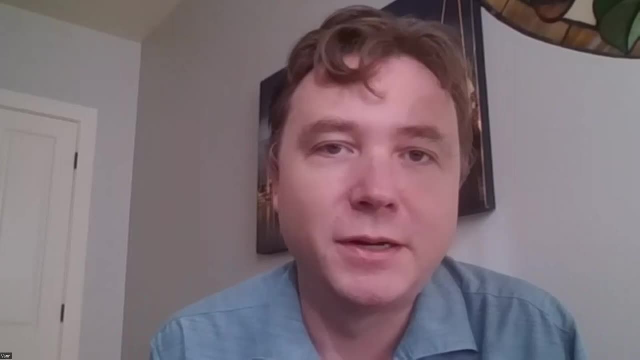 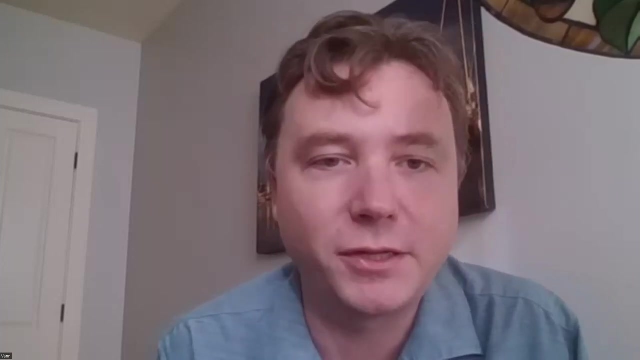 And I think one of the next things that we want to do here is really look in detail about the depositional environments versus the assemblages that we're seeing. But from the samples that have been selected, I'm not seeing big changes in the assemblage. 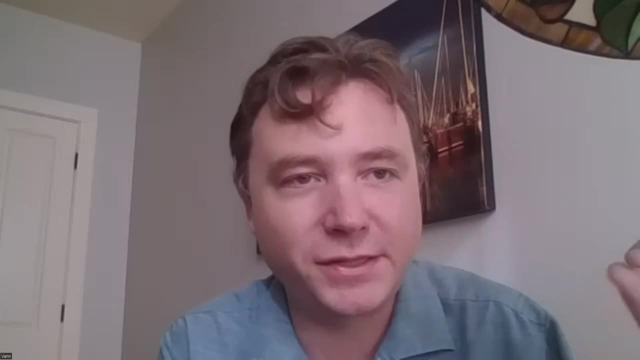 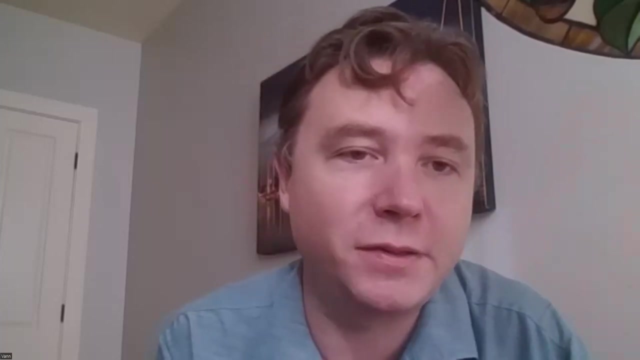 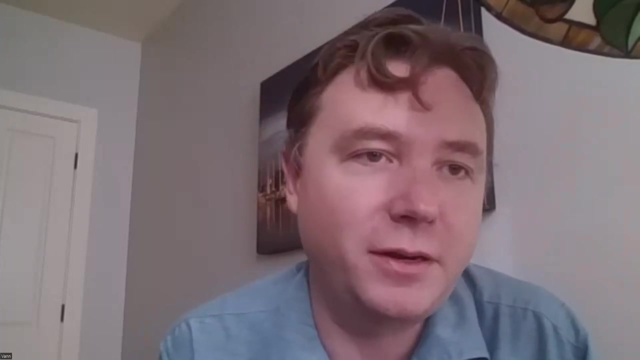 and relative abundance, So there's not some very distinct difference between some samples and others. There's some species that slowly come in and out and cyclic variations, which may be climatic or may be more controlled by whether it's an overbank deposit or different types of. 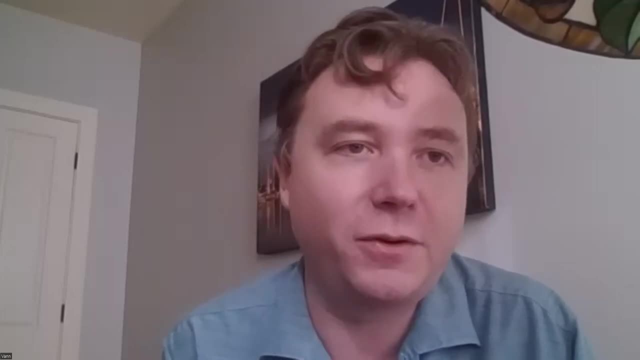 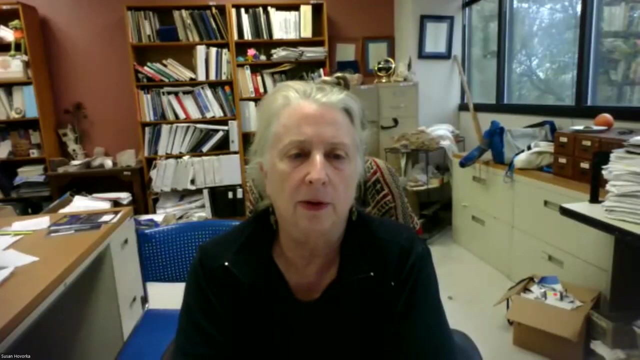 that, But that's something that we are definitely going to look in more detail at. You're not seeing evidence. You're not seeing evidence of big marine incursions going far up-dip. You're staying mostly in the fluvial, near shallow marine environment. 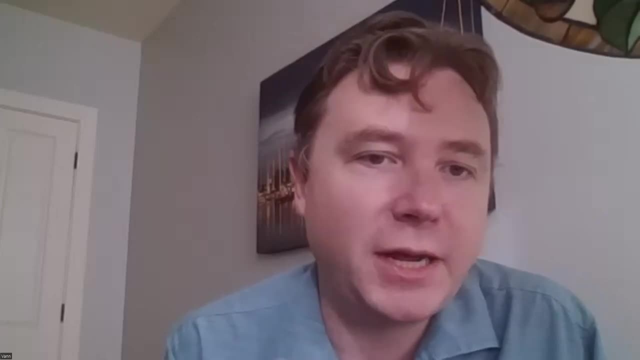 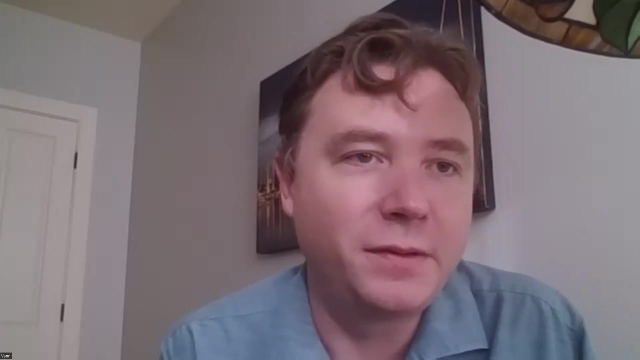 Yeah, well, we think it's fairly shallow, But the fact that we're seeing dinoflagellates in all of the samples and we're also seeing like rare nanos indicates that it's pretty marine. It's not like 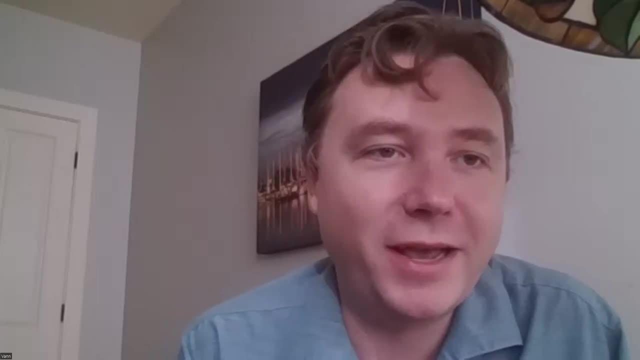 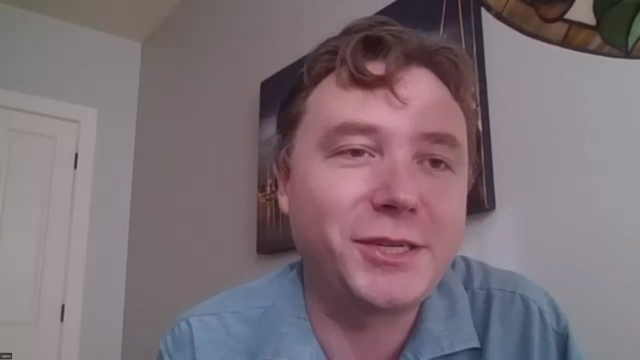 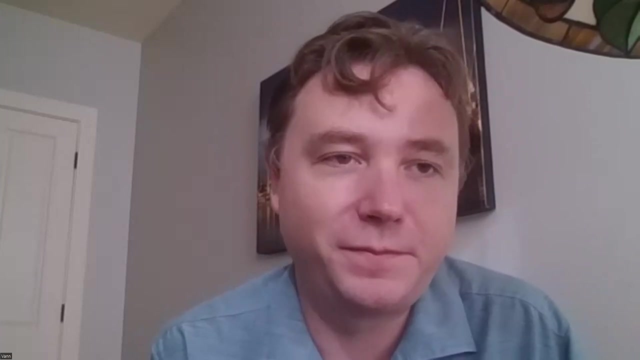 I hesitate to say with too much certainty because I don't want to step on the lithostratigraphy and the you know as possible interpretations, But it looks to us like shallow marine, but not super deep water. I want to know about the continuity of it. 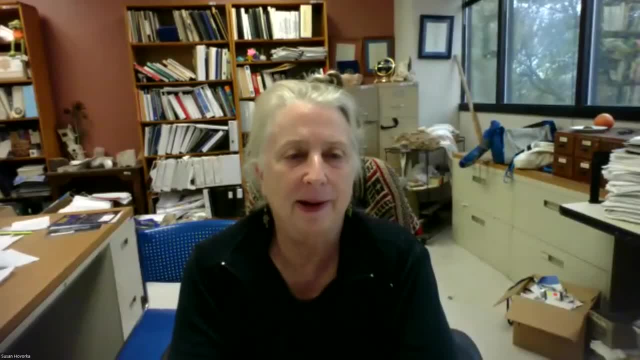 We want to know about the continuity of these units. So anything you guys have to say about that, tells us whether you would think they're continuous over miles, many miles. You know the lateral. Yeah, Yeah, Yeah, Yeah Yeah. 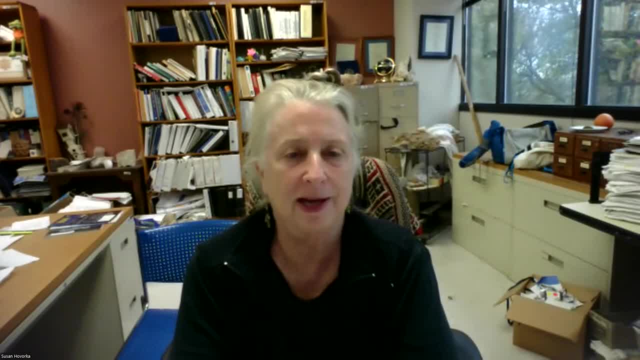 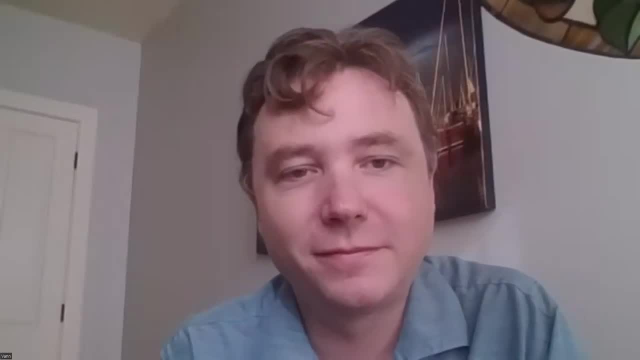 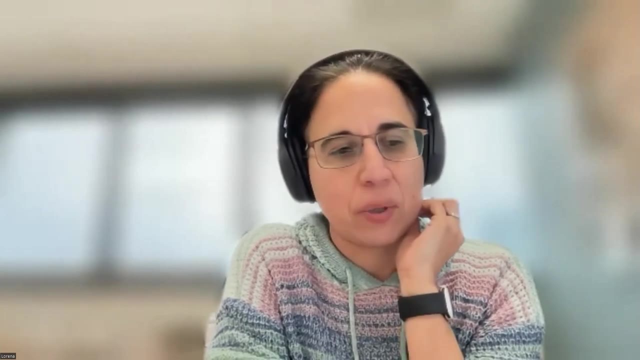 Yeah Yeah, The lateral continuity of those mud units is high value to our purposes, So that is critical information. Thanks, Yeah, Thank you. Thank you, Sue. I have a comment on that. That's part of the motivation with this work because especially in this area, we're in. 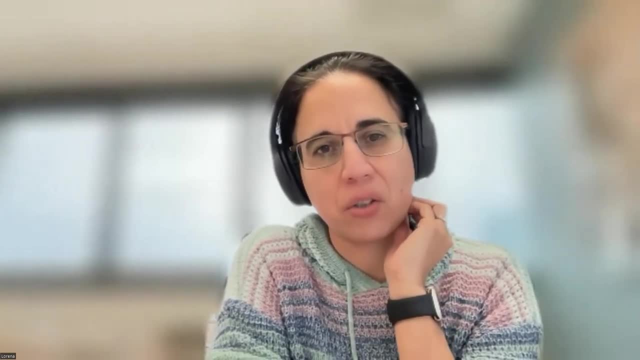 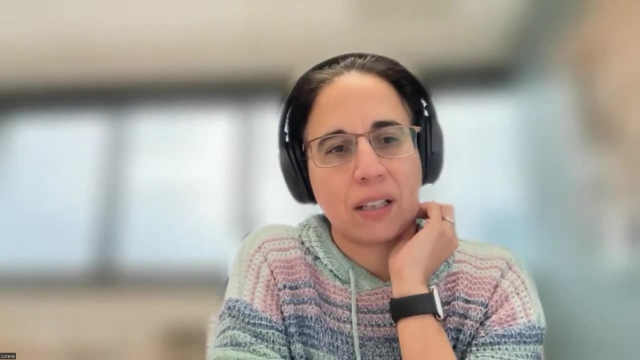 this growth fault region and it's very hard to make correlations between different fault blocks and also a long strike, I think with these two wells that Van was looking at Also. you know we're looking at at one point because they're very close to each other. 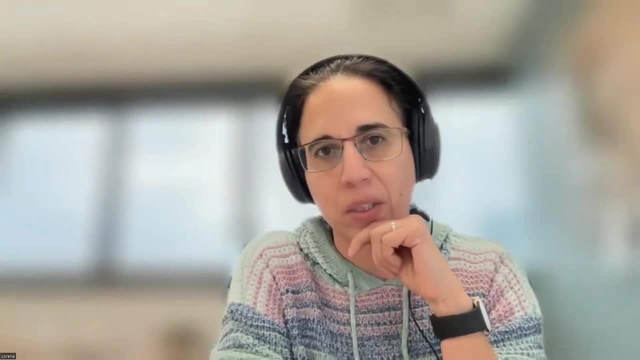 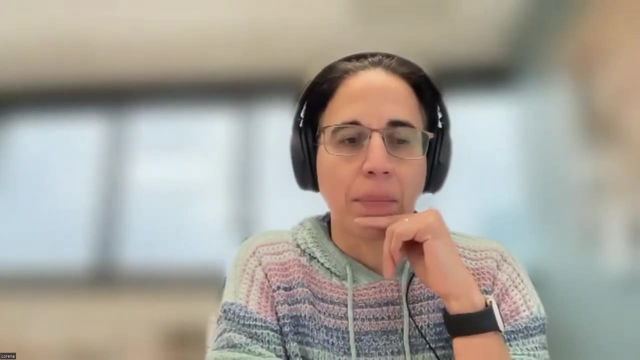 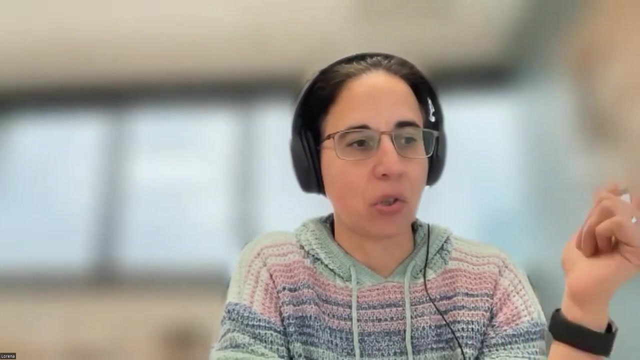 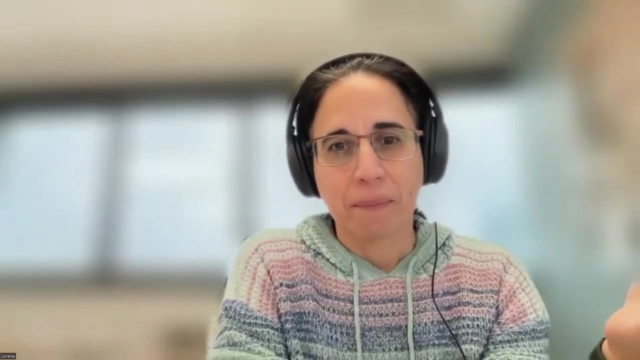 I think there is a whole lot more work that could be done, kind of like spreading the sampling along strike and along deep. So I mean the other thing is that beyond the age control and the paleoenvironmental interpretations, you know Van counted around 27,000 grains Van, is that correct? 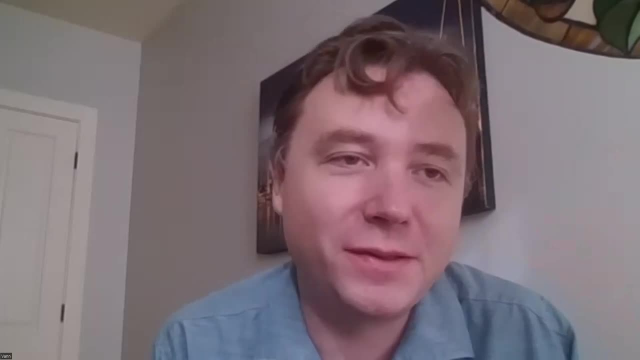 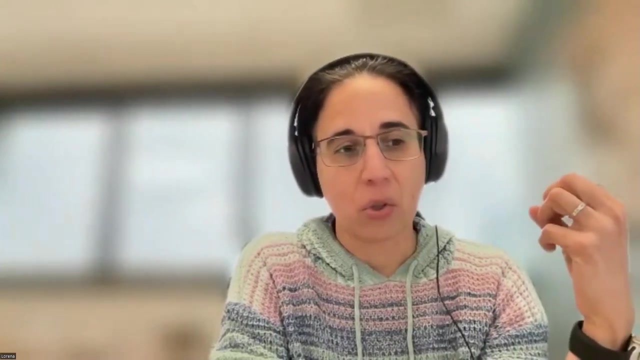 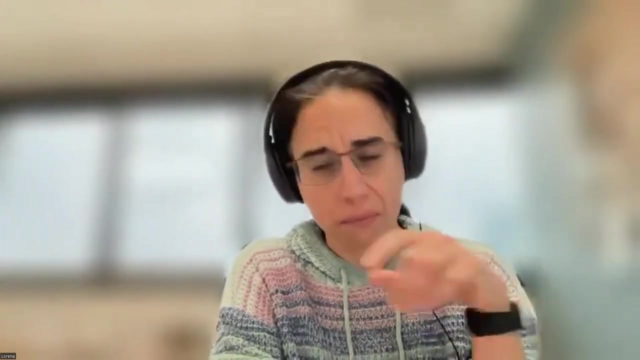 All over 23,000.. It sort of varied in their estimation, So that's a minimum. Yeah, So the value of this also is that it allows you to use relative abundances, And I think Dr Laurentiis is in the audience and we have been talking about using that. 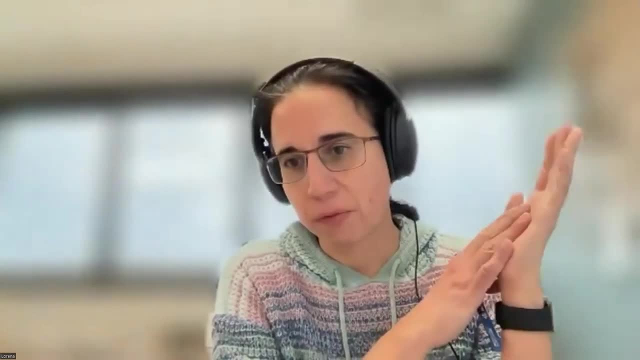 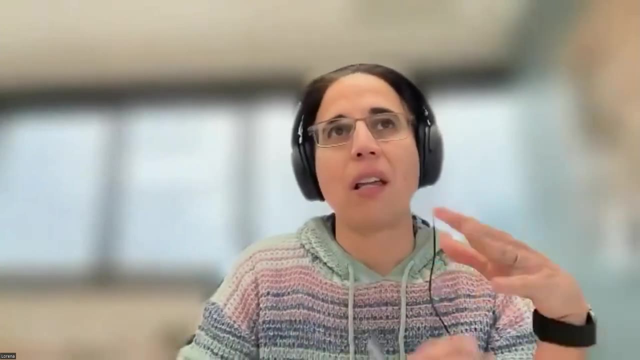 as well, to try to use it as a correlation tool if possible. It will tell us several things about paleoenvironments and age and everything, but also if we do it right in different sections, It could be a powerful tool for correlations, you know. 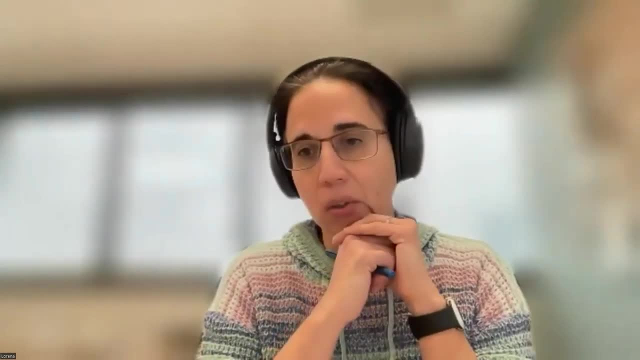 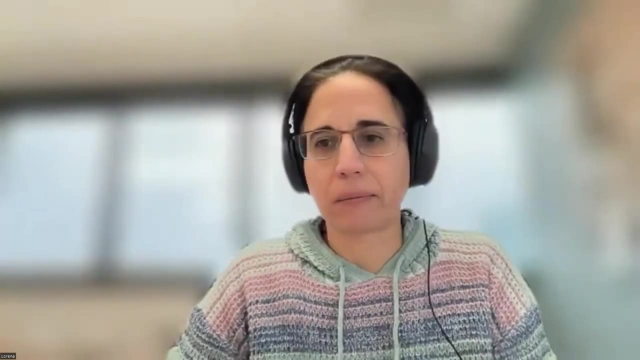 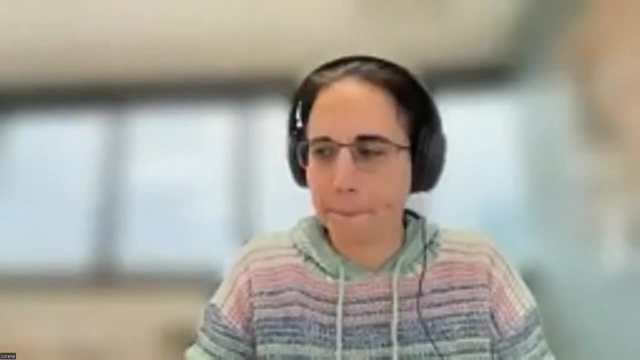 So yeah, as Van said, stay tuned, we'll see how that goes. But there is another question by Richard Dan. Richard, Hi, Good morning Van, Good talk, Good to hear some paleontology bandied about here. One comment like on the one thing with, especially with- Richard Howey. 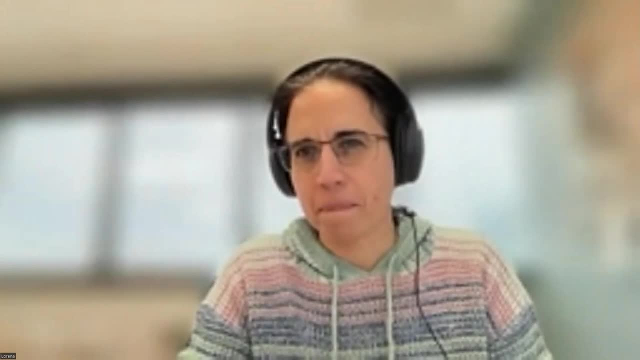 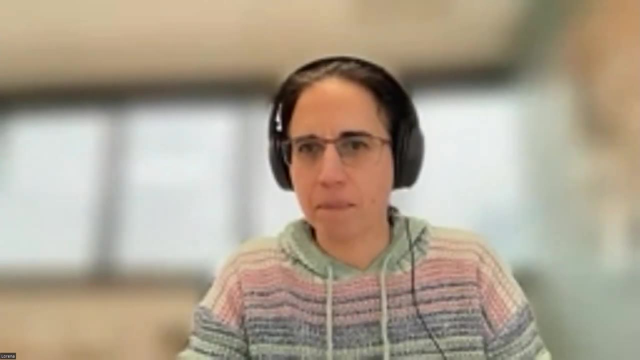 Yeah, Richard Howey is. when I was working at Exxon we were doing a lot of work in the- it'd be a slightly younger stuff- the Vicksburg-Frio play. A lot of that was counting nanofossils and tracking. 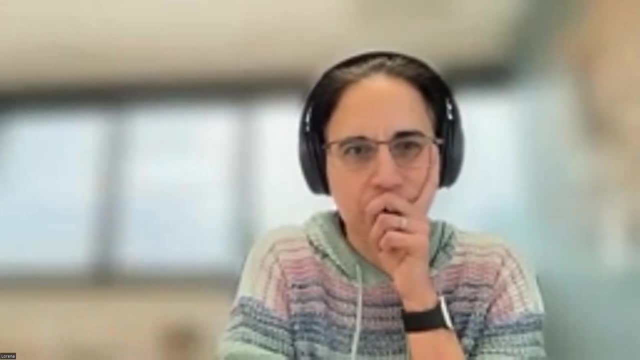 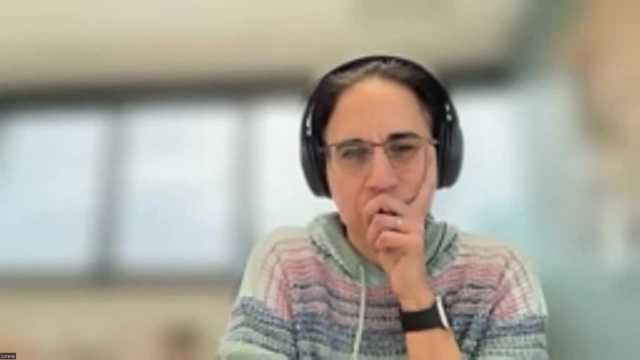 You could track really well with the sequence strat. It went really well with the sequence strat, tracking just the nano counts and seeing these bigger incursions, And then those were your good drapes, like you know what Sue was asking about. 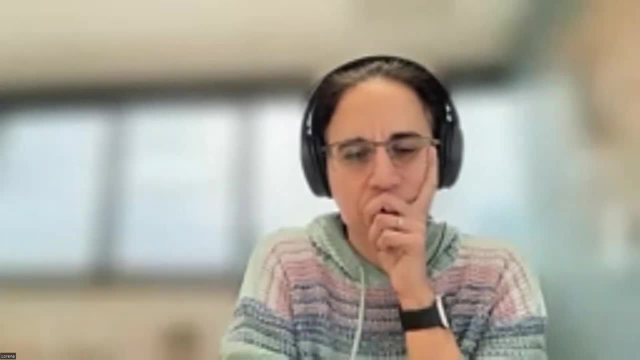 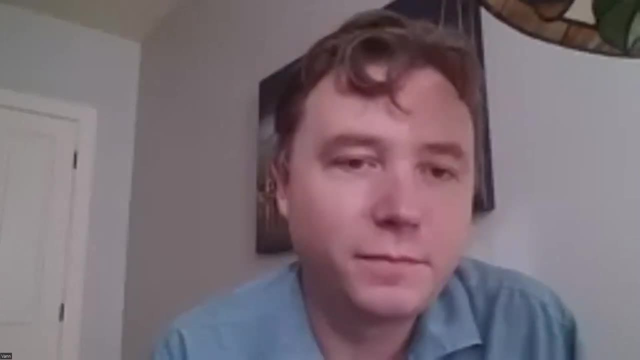 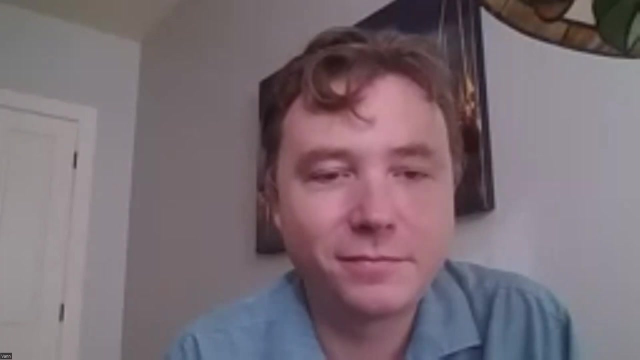 On the geochemistry. was that off of cuttings? No, that was only from the core. Okay, That's good, Because otherwise you're burying like uh, is that real or not? But okay, That's good. And I guess the other question I saw Neil Campion is on the thing- 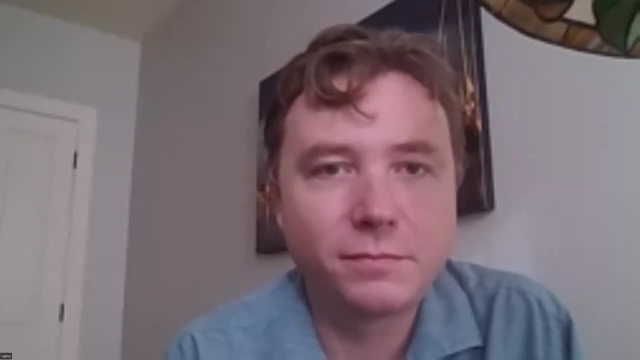 So whether or not you have talked to them, since they've done PetroStrat's done- an awful lot of work in the offshore environment, Um which I don't know if they've published any of that in any kind of um form or not. 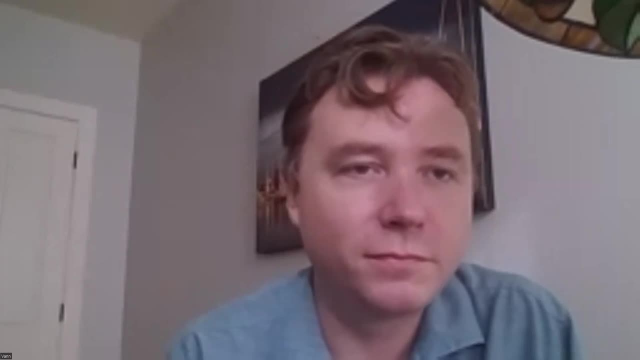 but I mean, that's what at Marathon- that's what I've relied heavily on- was was their work in combination with chemo strats um geochemical zonation. the two of them worked in tandem very well in in tracking these um units around. but obviously that was in. 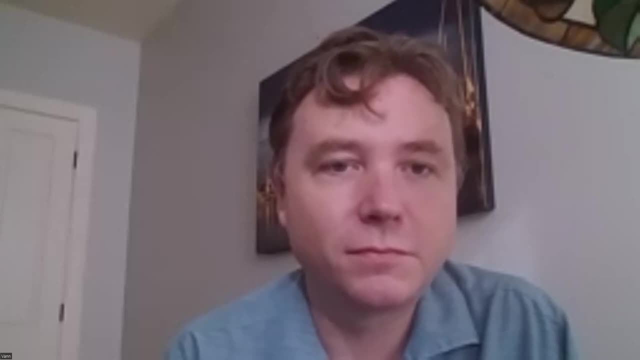 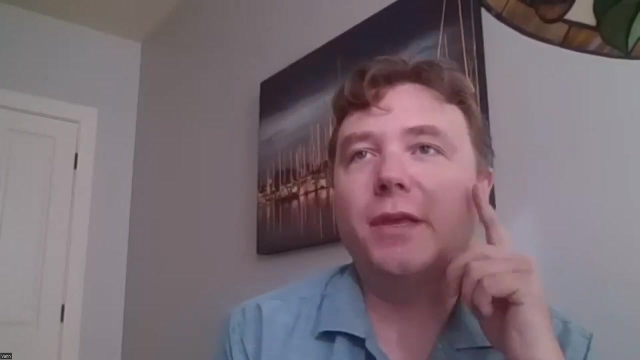 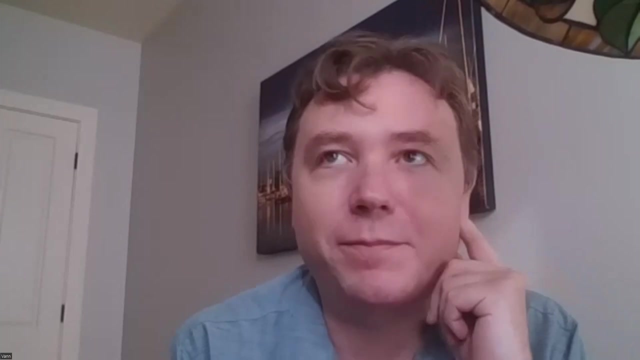 a much muddier environment than what you're dealing with. Okay, Yeah, Well, it um. our idea is that we, we like to, we think it's good that we're publishing this in an in sort of an open way, so that it's not like, uh, a black, a black box. 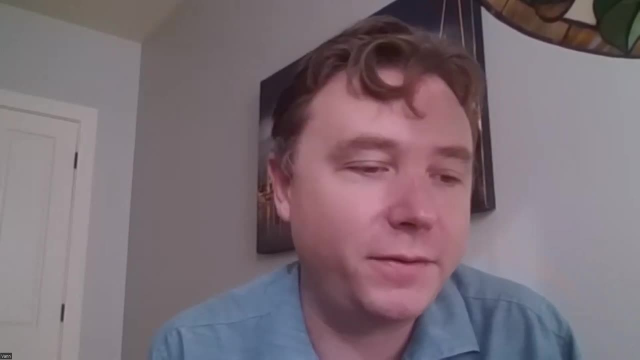 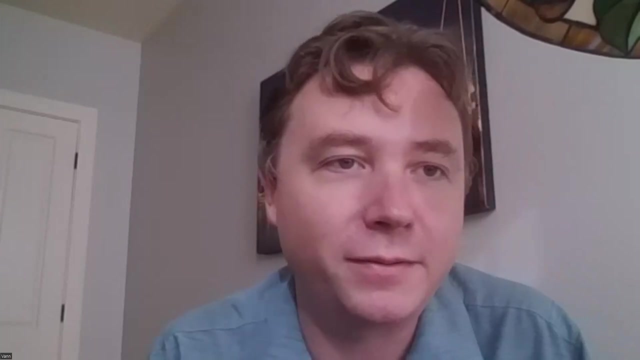 Right, So I'm trying to describe everything and and be, uh, very transparent here, And so hopefully we can get some more industry data, uh, into the public domain so we can, um, you know, get the academics involved with this biostratigraphic zonation. 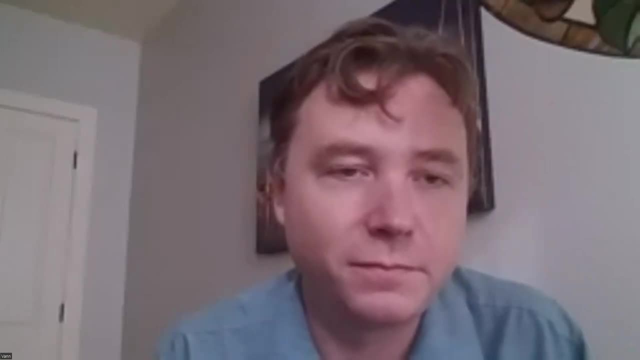 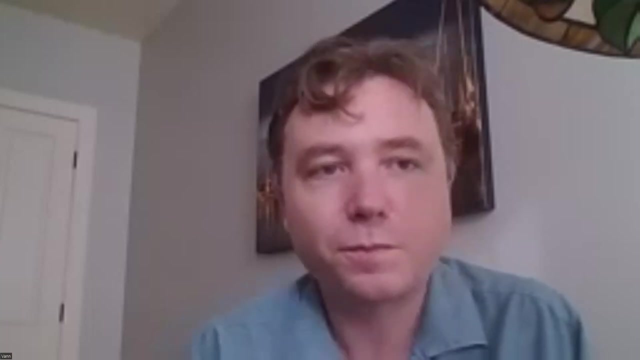 Was there anything? I mean I, although it looks like the BOEM has shut that down. they used to publish the actual data for a while. um, you know cause I cause, I would suspect. then some of the data that was collected may have gotten into the open, but whether that's 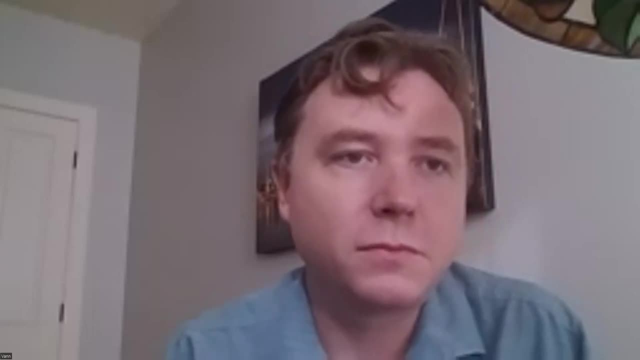 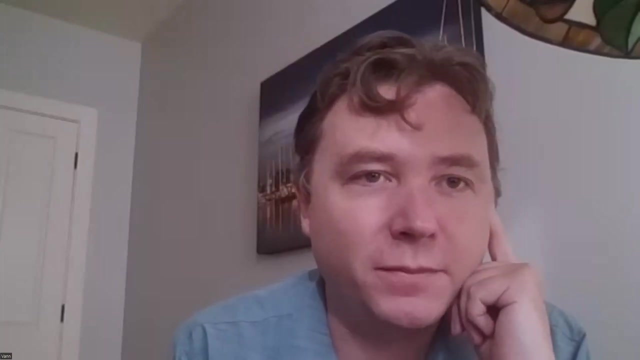 it, so it may still be out there somewhere where, even though it was petrostats, data may be public. Oh yeah, If I remember correctly, I think it's like 10 years and then it becomes public and you can request it. um, that's definitely an option to just like try to dig out all the publicly. 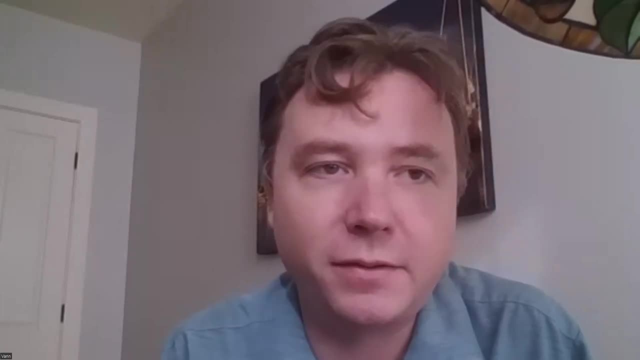 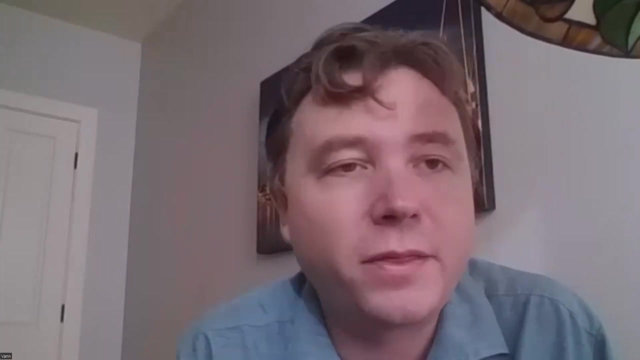 available BOEM, uh, PALI data and and do uh a zonation that way, use RASC. It's the same. It's a similar thing to what I did um with nanos in the Miocene. uh for that SEPM paper.